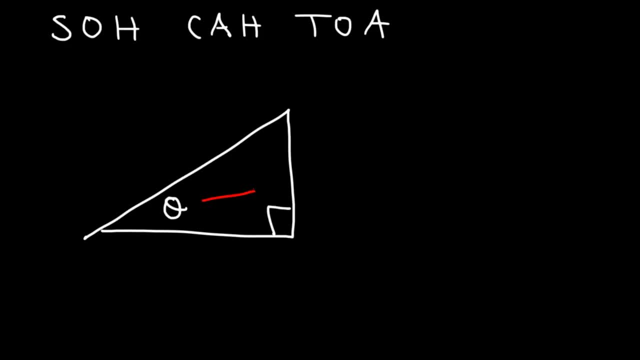 this triangle that you need to be familiar with. Opposites of theta: this is the opposite side and next to the angle, theta is the adjacent side and across the box or the right angle of the triangle, which is the hypotenuse That's. 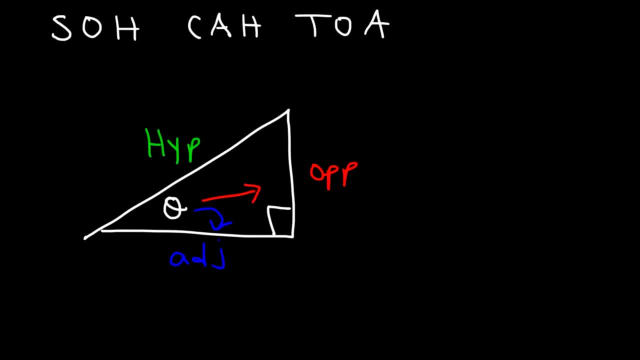 the longer side of the triangle. Now, if you recall, this is A, B and C. The Pythagorean theorem applies to right triangles: A squared plus B squared is equal to C squared. We're not going to focus on that too much, but 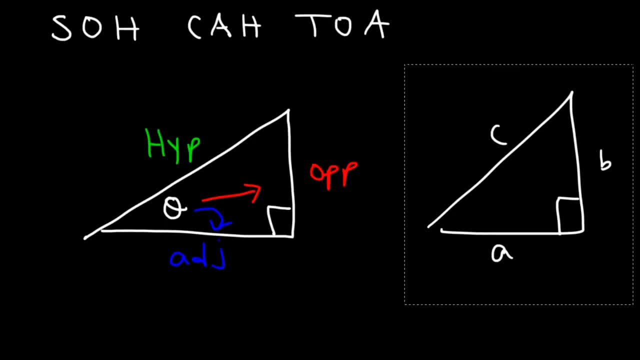 just be familiar with that equation. Now let's talk about the six trig functions in terms of sine, cosine, tangent, opposite, adjacent and hypotenuse Sine. theta according to SOH CAH TOA: s is for sine, o is for opposite, h is for hypotenuse Sine. 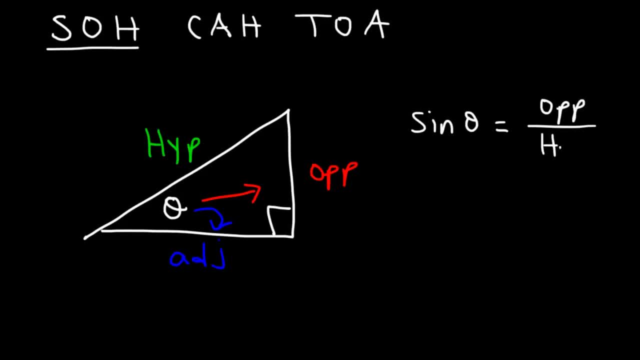 theta is equal to the opposite side divided by the hypotenuse Cosine. theta is equal to the opposite side divided by the hypotenuse 어�in theta is equal to the opposite side divided by the hypotenuse Dragons areלל uh. 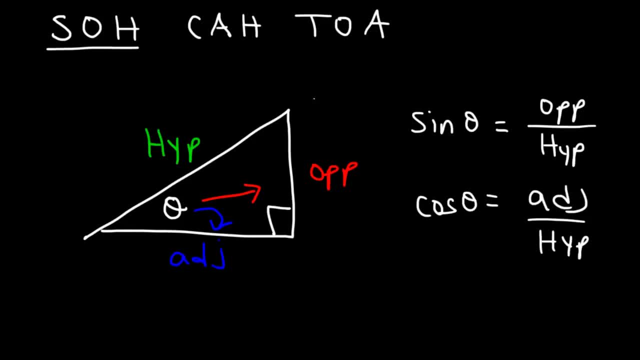 the adjacent side divided by the hypotenuse. Ka is for: cosine is adjacent over hypotenuse And tangent theta toa is equal to the opposite side divided by the adjacent side. So that's the tangent ratio. It's opposite over adjacent. Now we know that cosecant is 1 over sine, So cosecant. 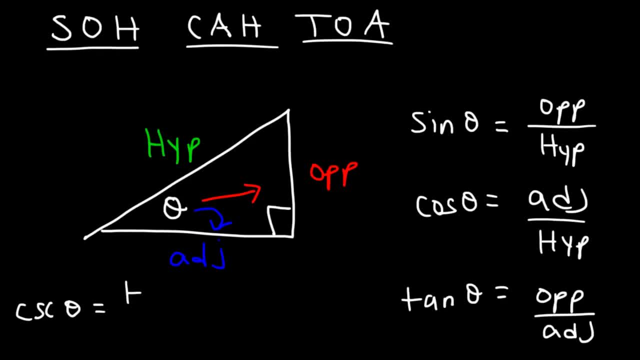 is basically hypotenuse divided by the opposite side. You just need to flip this particular fraction. Secant is the reciprocal of cosine, So secant is going to be hypotenuse divided by the adjacent side. Cotangent is the reciprocal of tangent, So if tangent is opposite over adjacent, 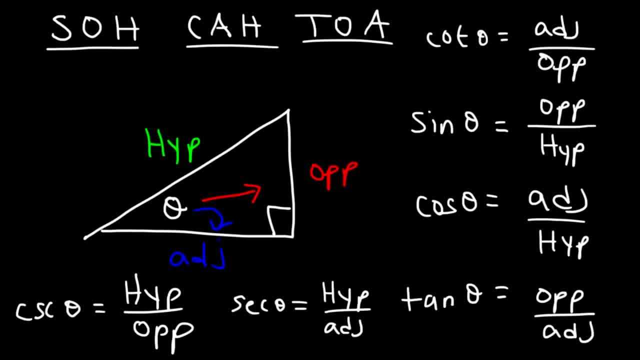 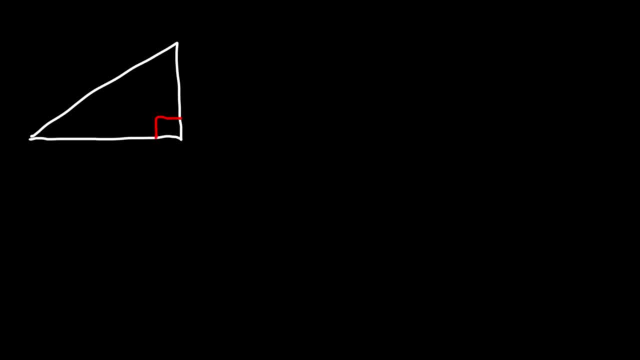 cotangent is adjacent divided by the opposite side. Now let's say, if we're given a ratio of cosine over cosine, So if we're given a ratio of cosine over cosine, a right triangle, and we have the value of two sides, Let's say this is 3 and this is 4.. 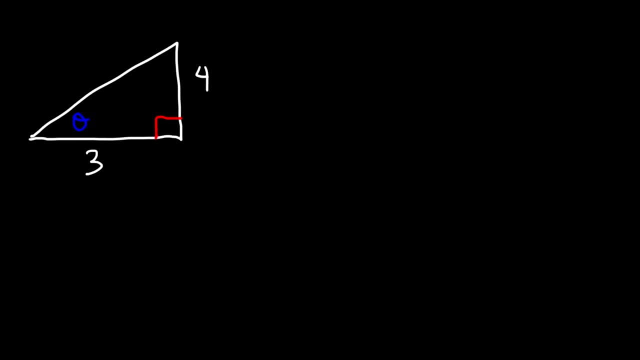 And here's the angle theta. Find the missing side of this right triangle and then find the values of all six trigonometric functions: Sine, cosine, tangent, secant, cosecant, cotangent. Now, to find the missing side, we need to use the Pythagorean theorem. 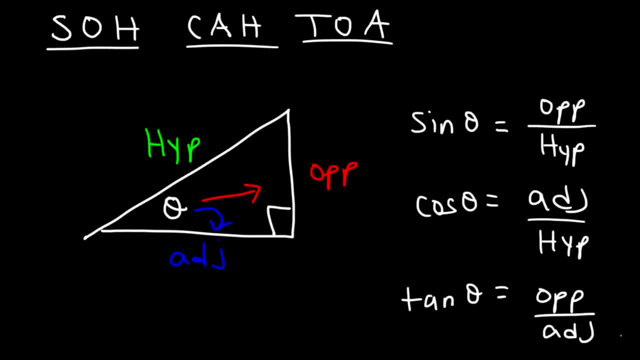 divided by the adjacent side. So that's the tangent ratio. It's opposite over adjacent. Now we know that cosecant is 1 over sine. so cosecant is basically hypotenuse divided by the opposite side. You just need to flip this particular fraction. Secant is the reciprocal of. 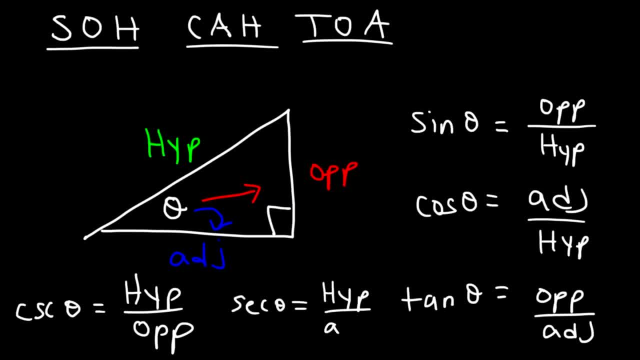 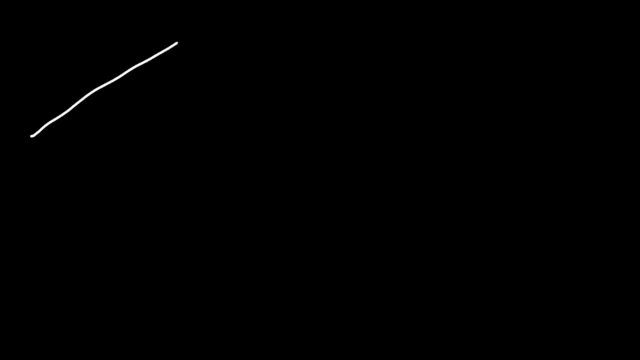 cosine. so secant is going to be hypotenuse divided by the adjacent side. Cotangent is the reciprocal of tangent. so if tangent is opposite over adjacent, cotangent is adjacent divided by the opposite side. Now let's say, if we're given a right triangle and we have the value of two, 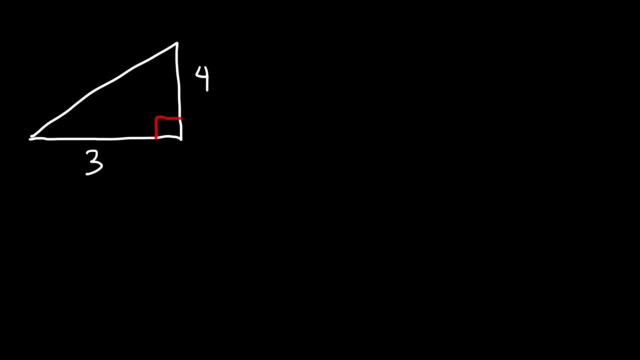 sides. Let's say this is 3 and this is 4, and here's the angle theta. Find the missing side of this right triangle and then find the values of all six trigonometric functions: Sine, cosine, tangent, secant, cosecant, cotangent. Now to find the missing. 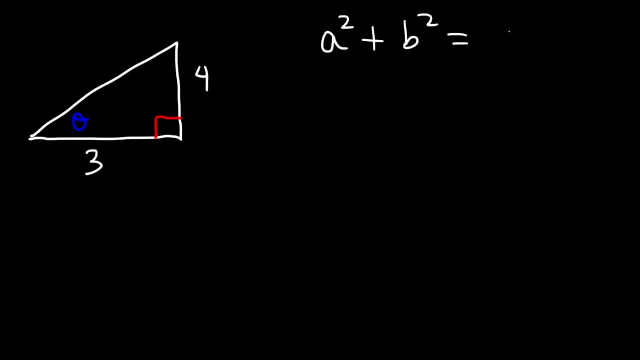 side, we need to use the Pythagorean theorem: a squared plus b squared is equal to c squared. So a is 3, b is 4.. And we got to find the missing side, c, which is the hypotenuse: 3 squared is 9, 4 squared is 16.. 9 plus 16 is 25.. And if 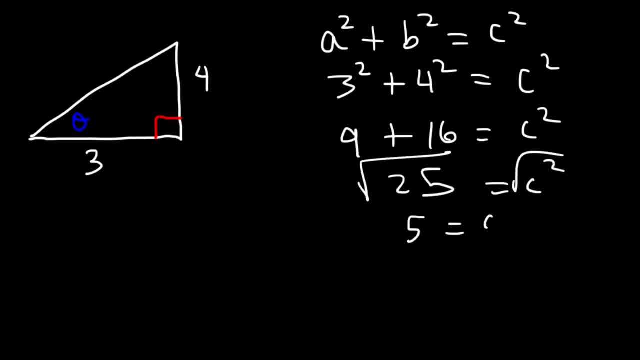 you take the square root of both sides, you can see that the hypotenuse is 5.. Now it turns out that there are some special numbers. There's the 3,, 4,, 5 right triangle, the 5,, 12,- 13 right triangle, the 8,, 15,. 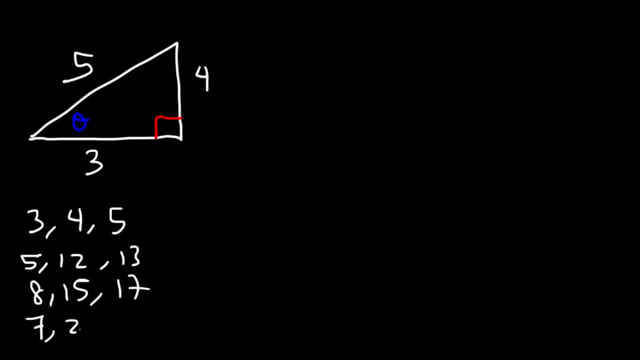 17 right triangle and the 7,, 24,, 25 right triangle, And any whole number, ratios or multiples of these numbers will also work. For example, if we multiply this by 2,, we'll get 6,, 8,, 10.. That can also work. Or if you multiply it by 3,, you get the 9,, 12,. 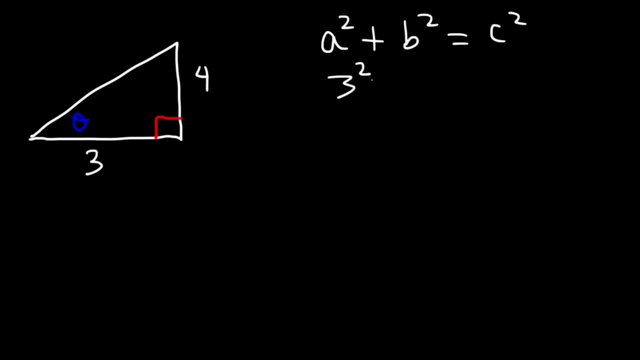 a squared plus b squared is equal to c squared. So a is 3,, b is 4.. And we've got to find the missing side c, which is the hypotenuse. 3 squared is 9,, 4 squared is 16.. 9 plus 16 is 25.. And if you take the square root of both sides, 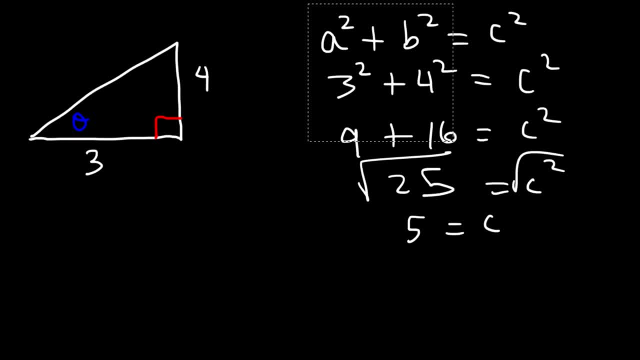 you can see that the hypotenuse is 5.. Now it turns out that there are some special numbers. There's a 3,, 4, and 5. And if you take the square root of both sides, you can see that the hypotenuse is 5.. 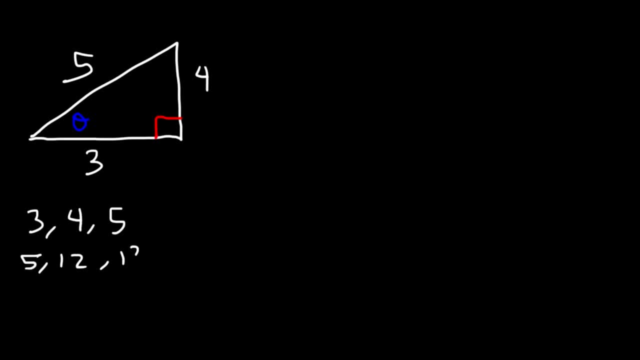 3,, 4, 5 right triangle, the 5,, 12, 13 right triangle, the 8,, 15,, 17 right triangle and the 7,, 24, 25 right triangle And any whole number, ratios or multiples of these numbers will also work. 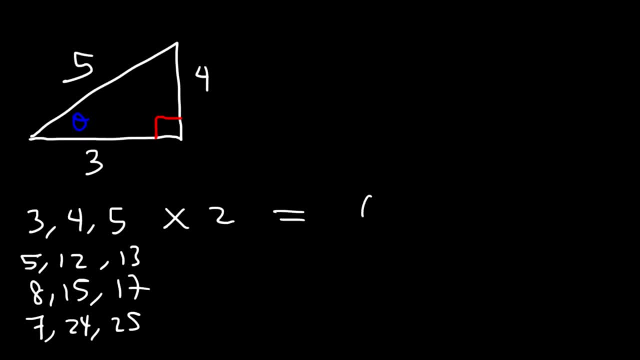 For example, if we multiply this by 2,, we'll get 6,, 8,, 10.. That can also work. Or if you multiply it by 3,, you get the 9,, 12,, 15.. If you multiply this one by 2,, you get the 10,, 24,, 26 triangle. 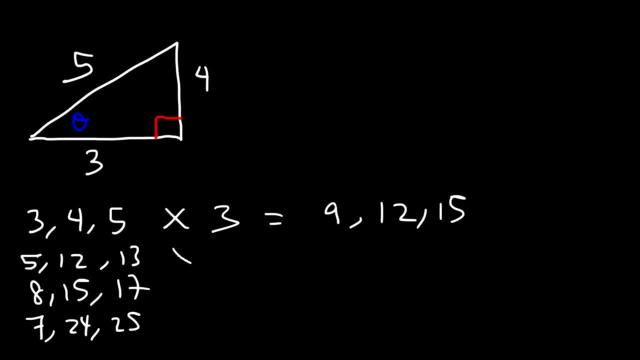 Those are also special triplets. They work with any right triangle. Now some other numbers that are less common but you might see are the 9, 40, 41 triangle and the 11,, 60, 61. So if you see some of these numbers, you can find the missing side quickly if you know them. 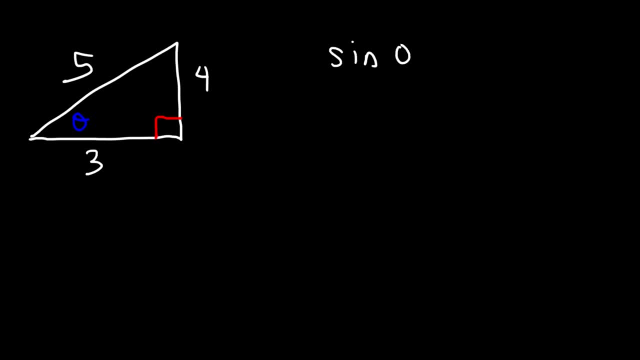 So now let's finish this problem. So what is the value of sine theta? So, according to Sokotoa, we know that sine theta is equal to the opposite side divided by the adjacent side In the part. SOH Opposite to theta is 4.. 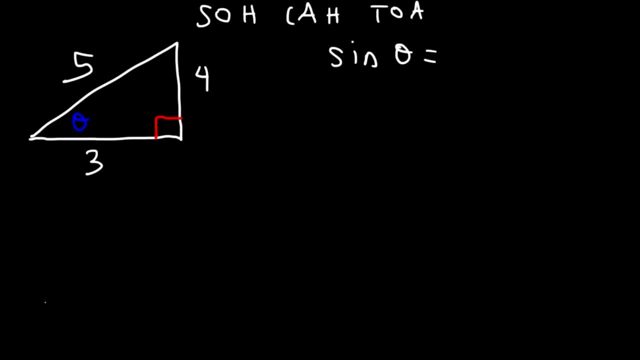 And hypotenuse is 5.. So therefore sine theta is going to be 4 divided by 5.. Now cosine theta is equal to the adjacent side divided by the hypotenuse. So we said 4 is the opposite side, 5 is the hypotenuse and 3 is the adjacent side. 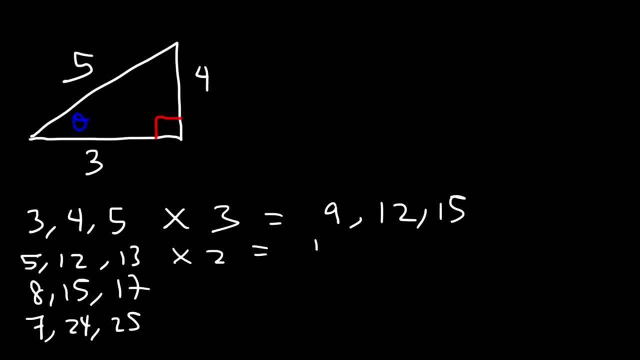 15 triangle. If you multiply this one by 2, you get the 10,, 24, 26 triangle. Those are also special triplets. They work with any right triangle. Now some other numbers that are less common but you might see are the 9,, 40,, 41 triangle. 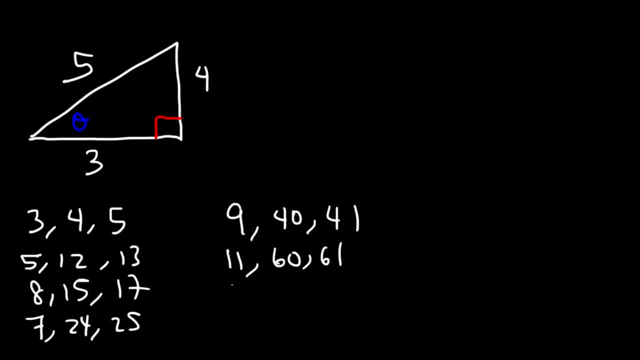 and the 11,, 60, 61. So if you see some of these numbers, you can find the missing side quickly if you know them. So now let's finish this problem. So what is the value of sine theta? So, according to SOHCAHTOA, we know that sine theta is equal to the opposite side. 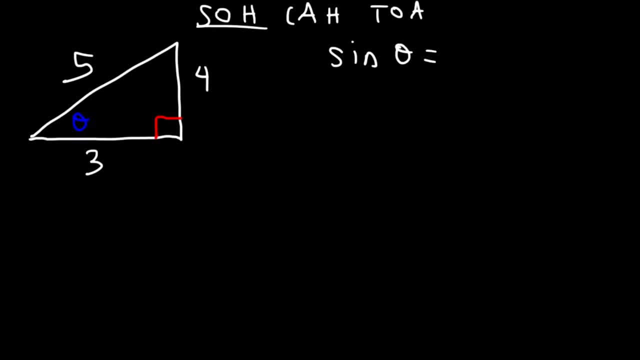 divided by the adjacent side in the part SOH Opposite to theta is 4 and hypotenuse is 5.. So therefore, sine theta is going to be 4 divided by 5.. Now cosine theta is equal to the adjacent side divided by the hypotenuse. 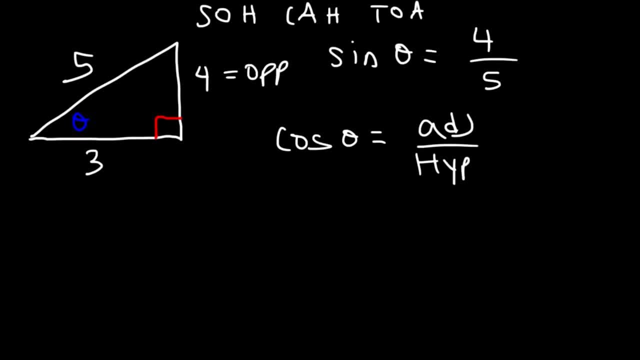 So we said 4 is the opposite side, 5 is the hypotenuse and 3 is the adjacent side. So in this case it's going to be 3 divided by 5.. So that's the value of cosine. Now let's find the value of tangent Tangent theta according to TOA. 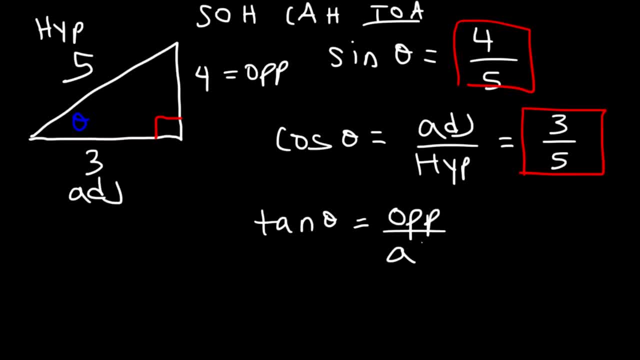 is equal to the opposite side divided by the adjacent side. So that's going to be 4 divided by 3.. So that's the value of tangent. Now, once we have these three, we can easily find the other three. To find cosecant, it's 1 over sine, so just. 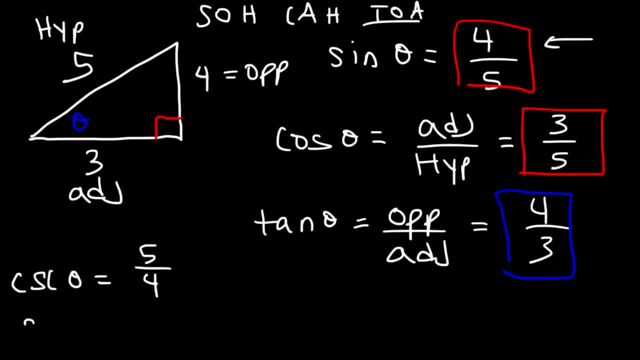 flip this fraction, It's going to be 5 over 4.. And secant is the reciprocal of cosine. so flip this fraction. Secant is going to be 5 over 3.. Cotangent is the reciprocal of tangent. So if cotan, I mean if tangent- is 4 over 3, cotangent is 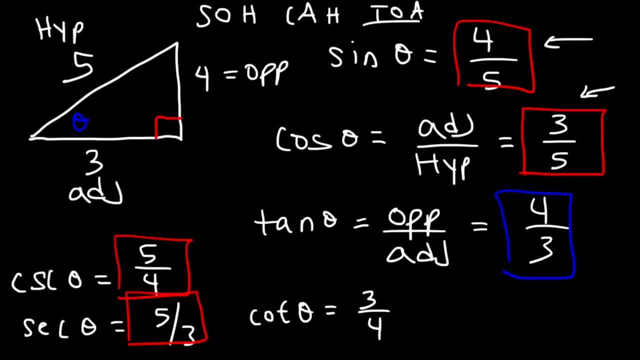 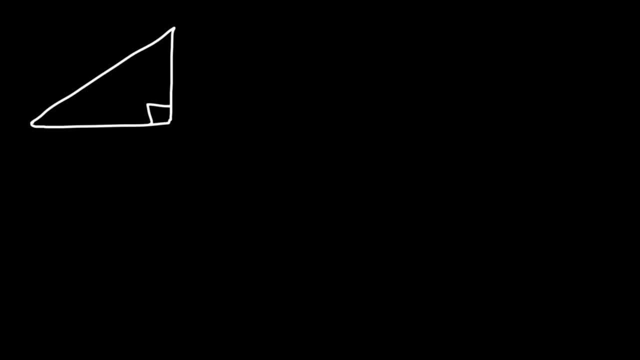 going to be 3 over 4.. And that's how you could find the value of the six trigonometric functions. So let's say this is theta again, and this side is 8, and this side is 17.. Find the missing side and then use the completed triangle to find the value of. 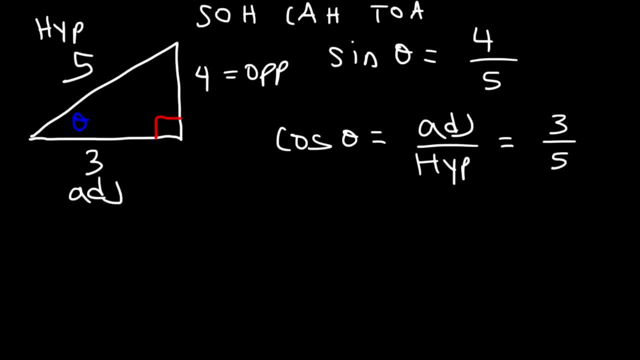 So in this case it's going to be 3 divided by 5.. So that's the value of cosine. Now let's find the value of tangent. Tangent theta, according to Toa, is equal to the opposite side divided by the adjacent side. 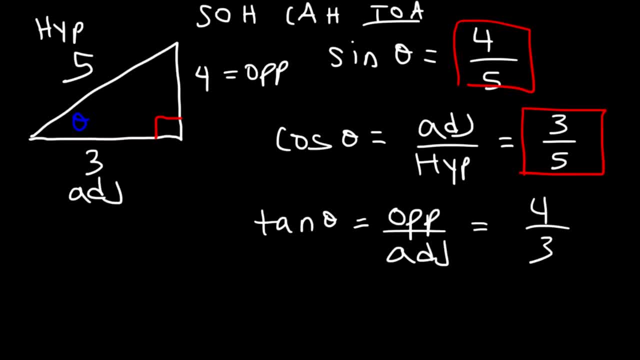 So that's going to be cosine. So that's the value of tangent. Now, once we have these three, we can easily find the other three. To find cosecant, it's 1 over sine. so just flip this fraction, It's going to be 5 over 4.. 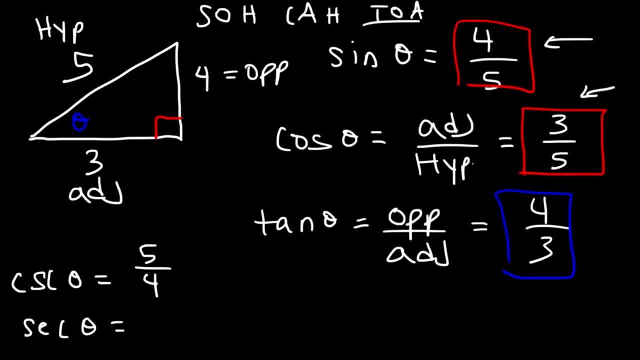 And secant is the reciprocal of cosine. so flip this fraction. Secant is going to be 5 over 3.. Cotangent is the reciprocal of tangent. So if tangent is 4 over 3, cotangent is going to be 3 over 4.. 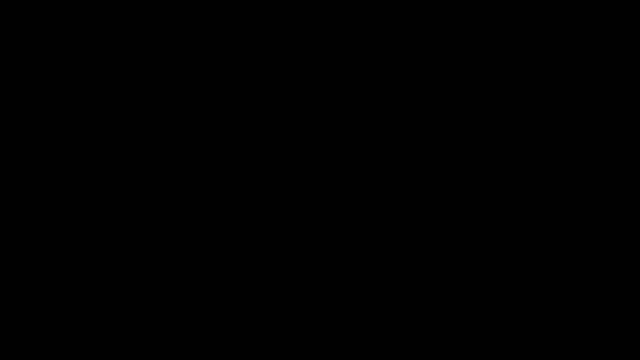 And that's how you could find the value of the six trigonometric functions. Let's try another problem. So let's say this is theta again, And this side is 8, and this side is 17.. Find the missing side and then use the completed triangle to find the value of the six trigonometric functions. 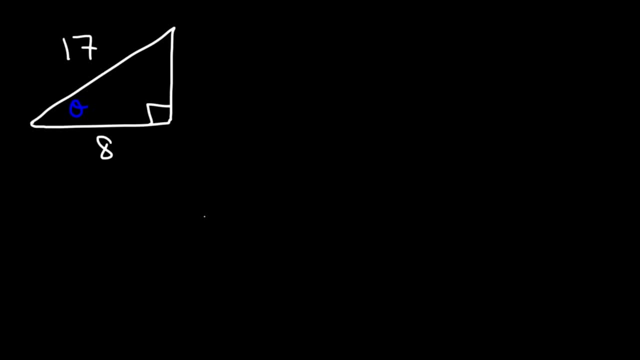 So go ahead and pause the video and work on this problem. So first we need to know that this is the 8, 15, 17 triangle. If you ever forget, you can fall back to this equation. So a is 8.. 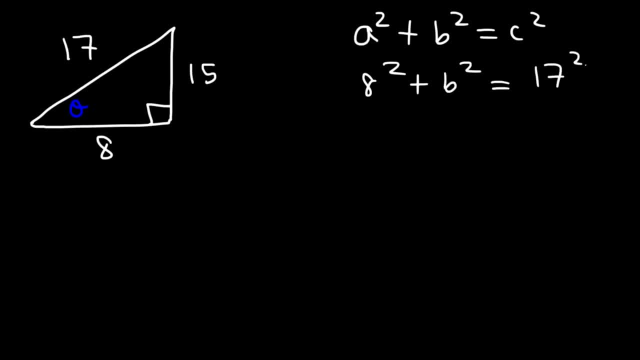 We're looking for the missing side b and the hypotenuse is 17.. 8 squared is 64.. And 17 squared is 289.. 289 minus 64 is 225.. And we need to take the square root of both sides. 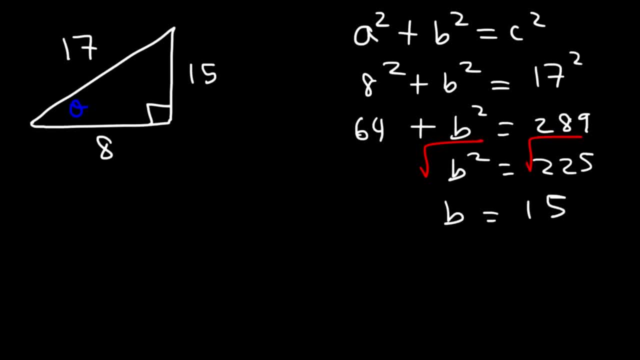 And the square root of 225 is 15, which gives us the missing side of the triangle. So now Go ahead and find the value of sine theta, cosine theta, tangent theta, and then cosecant theta, secant theta and cotangent theta. 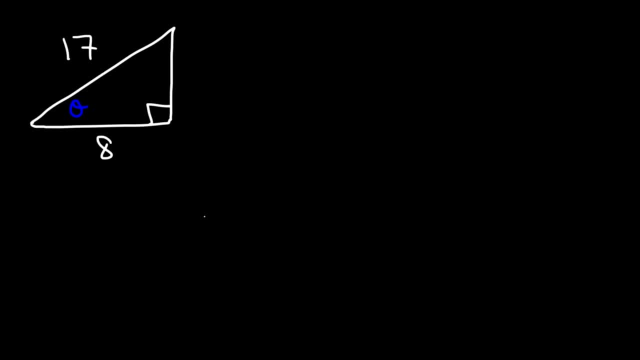 the six trigonometric functions. So go ahead and pause the video and work on this problem. So first we need to know that this is the 8,, 15, 17 triangle. If you ever forget, you can fall back to this equation. 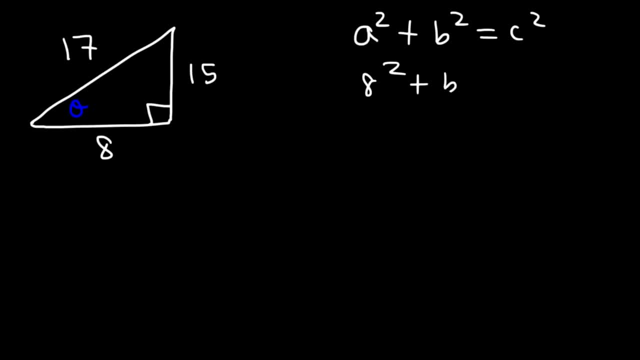 So a is 8,. we're looking for the missing side b and the hypotenuse is 17.. 8 squared is 64, and 17 squared is 289.. 289 minus 64 is 225.. And we need to take the square root of. 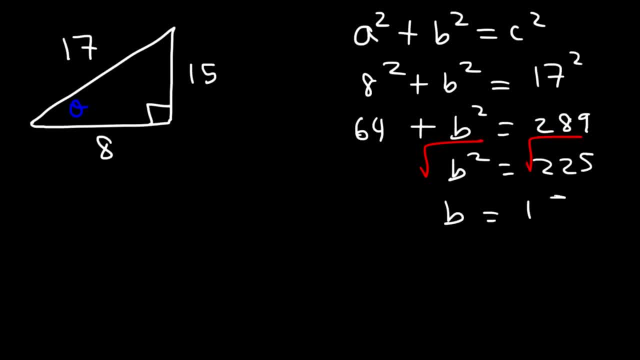 both sides, and the square root of 225 is 15,, which gives us the missing side of the triangle. So now go ahead and find the value of sine theta, cosine theta, tangent theta, and then cosecant theta, secant theta and cotangent theta, So using SOHCAHTOA. 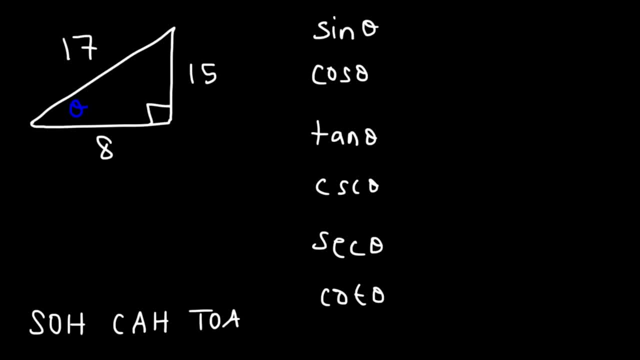 we know that sine is equal to the opposite side divided by the hypotenuse. So let's label all the three sides: 17 is the hypotenuse, 8 is the adjacent side and opposite to theta is 15.. So opposite over hypotenuse, this is going to be 15 divided by 17.. So that is the. 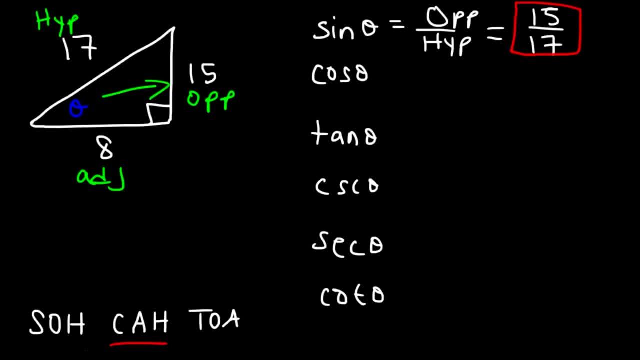 value of sine theta. Now cosine theta is going to be equal to the adjacent side divided by the hypotenuse. So the adjacent side is 8, the hypotenuse is 17.. So cosine theta is 8 over 17.. Tangent, based on TOA is going to be opposite over. 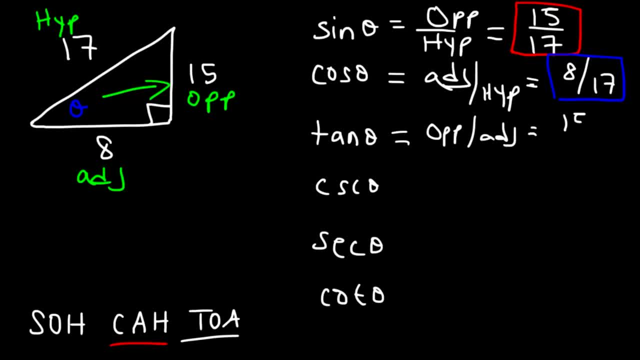 adjacent. So opposite is 15, adjacent is 8.. Therefore, tangent is going to be 15 divided by 8.. Now, cosecant is the reciprocal of sine. So if sine theta is 15 over 17,, cosecant is going to be 17 over 15.. Secant is the reciprocal of. 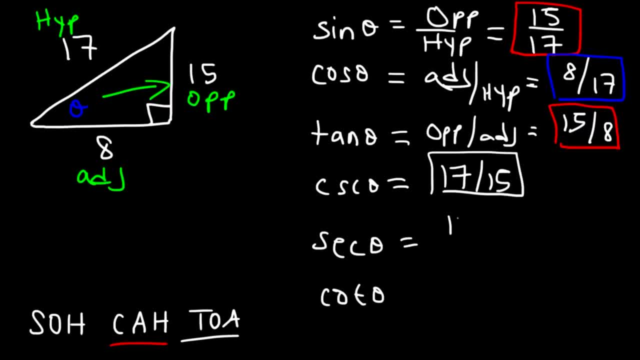 cosine. So if cosine is 8 over 17,, secant is 17 over 8.. You just got to flip it And cotangent is the reciprocal of tangent. So cotangent is going to be 8 over 15.. Just flip this fraction And now we have the values of the six trigonometric. 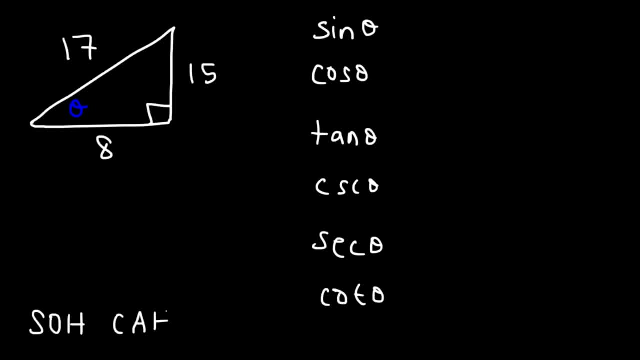 So, using SOHCAHTOA, we know that sine is equal to the opposite side divided by the hypotenuse. So let's label all the three sides: 17 is the hypotenuse, 8 is the adjacent side, And opposite to theta is 15.. 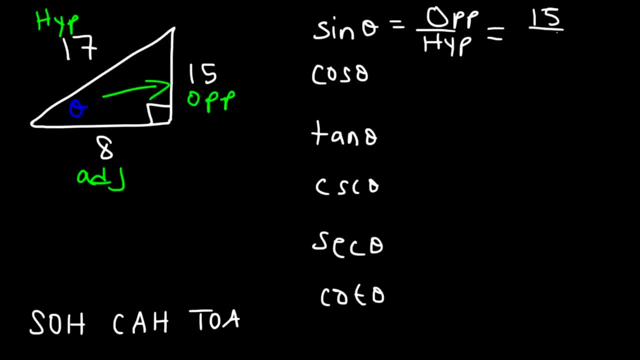 So opposite over hypotenuse. This is going to be 15 divided by 17.. So that is the value of sine theta. Now cosine theta is going to be equal to the adjacent side divided by the hypotenuse. So the adjacent side is 8.. 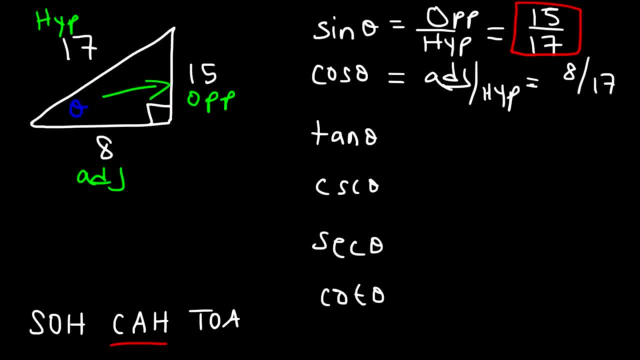 The hypotenuse is 17.. So cosine theta is 8 over 17.. Tangent Based on TOA, it's going to be opposite over adjacent. So opposite is 15, adjacent is 8.. Therefore, tangent is going to be 15 divided by 8.. 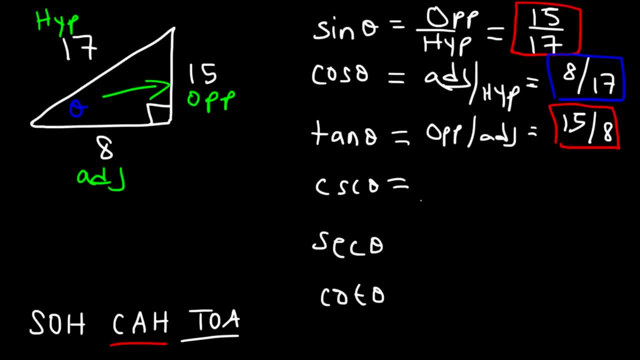 Now, cosecant is the reciprocal of sine. So if sine theta is 15 over 17,, cosecant is going to be 17 over 15.. Secant is the reciprocal of cosine. So if cosine is 8 over 17,, secant is 17 over 8.. 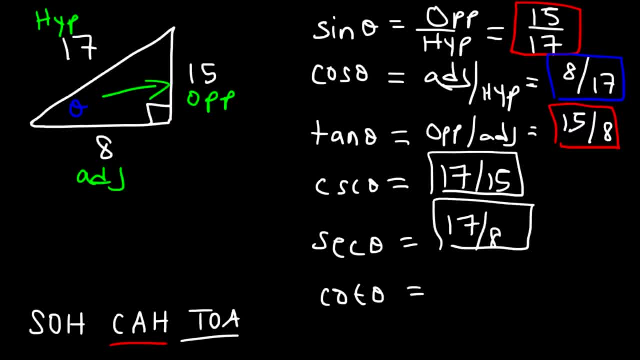 You just got to flip it, And cotant is the reciprocal of tangent, So cotangent is going to be 8 over 15.. Just flip this fraction And now we have the values of the six trigonometric functions, And that's all you got to do. 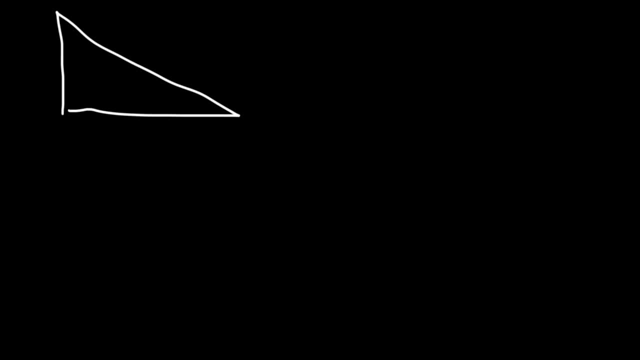 So here's a different problem. So let's say, here's our right angle, And this time this is theta And let's say the hypotenuse is 25. And this side is 15. Find the missing side And then go ahead and find the value of the six trigonometric functions. 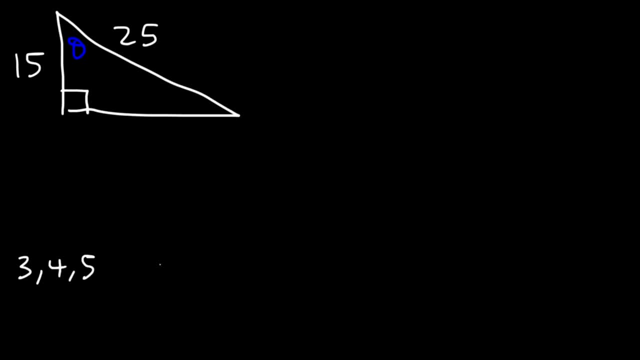 So this is going to be similar to the 3,, 4, 5 triangle. Notice that if we multiply everything by 5, we'll get two of the three numbers that we need. 3 times 5 is 15.. 4 times 5 is 20.. 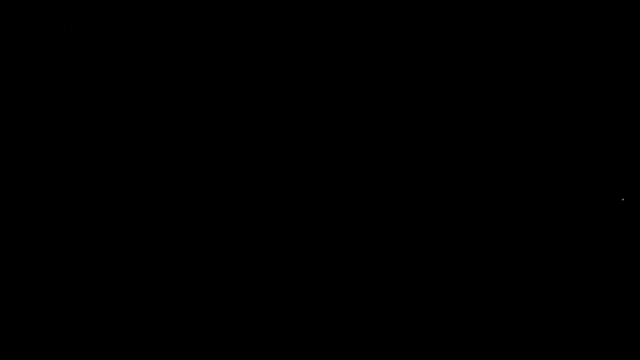 functions And that's all you got to do. So here's a different problem. So let's say: here's our right angle, And this time this is theta. And let's say: the hypotenuse is 25 and this side is 15.. Find the missing side and then go ahead. 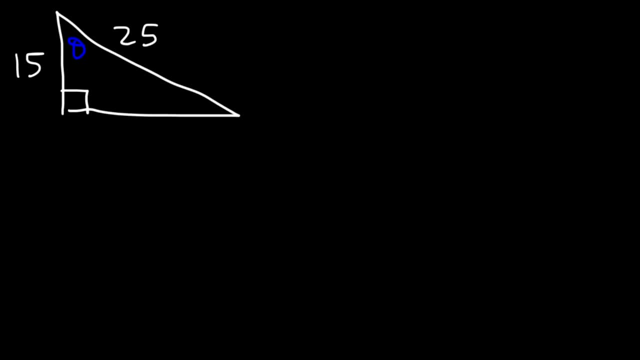 and find the value of the six trigonometric functions. So this is going to be similar to the 3,, 4, 5 triangle. Notice that if we multiply everything by 5, we'll get two of the three numbers that we need. 3 times 5 is. 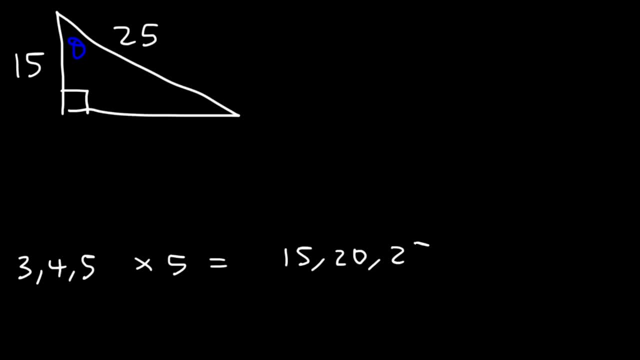 15.. 4 times 5 is 20.. 5 times 5 is 25.. So we have the 15 and we have the 25.. Therefore, the missing side must be 20.. And you can use the Pythagorean Theorem to confirm this if you want to. 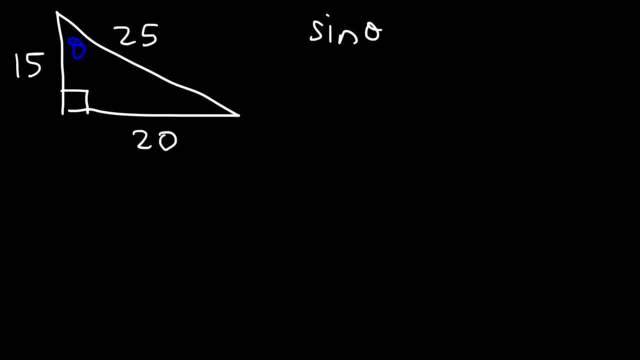 So now let's go ahead and find the value of sine theta. So opposite to theta is 20.. The hypotenuse is always across the box, It's the longer side. So 27 is the hypotenuse, And adjacent to 15, or right next to it is 15.. I mean adjacent to theta is 15.. So this: 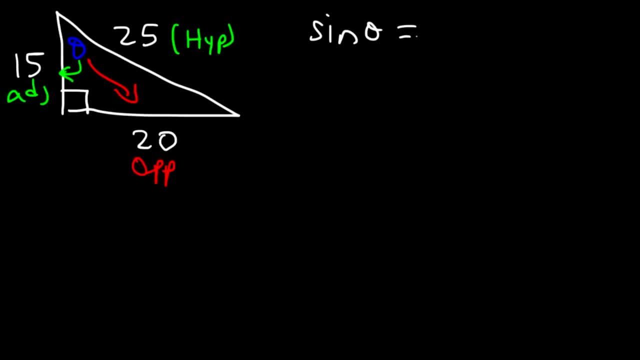 is the hypotenuse- Now, sine theta, we know it's opposite- divided by hypotenuse. So it's 20 over 25, which reduces to 4 over 5 if we divide both numbers by 5.. 20 divided by 5. 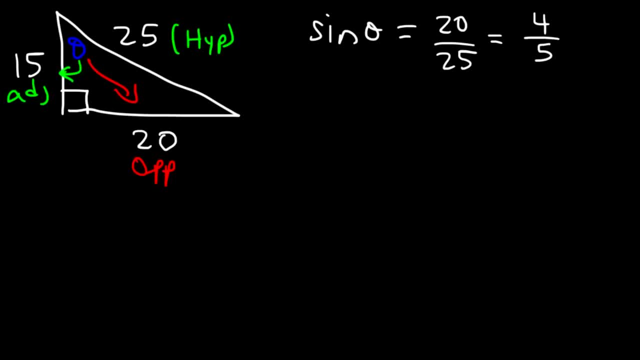 is 4.. 25 divided by 5 is 5.. Cosine theta is adjacent over hypotenuse, So that's 15 divided by 25, which reduces to 3 divided by 5.. Cosine theta is opposite over adjacent, So 20 over 15, which becomes if you divide by. 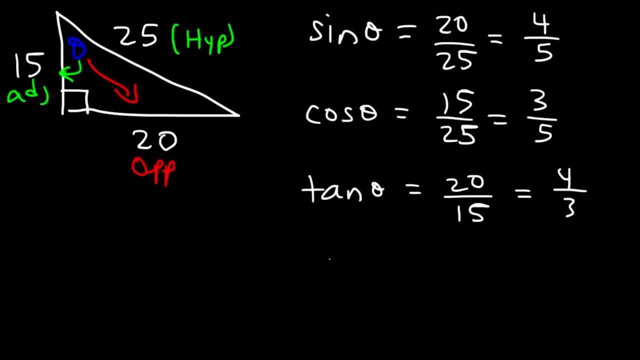 5, that's going to be 4 over 3.. Now, cosecant is the reciprocal of sine, so it's going to be 5 over 4, based on this value, And if cosine is 3 over 5, then secant, the reciprocal of. 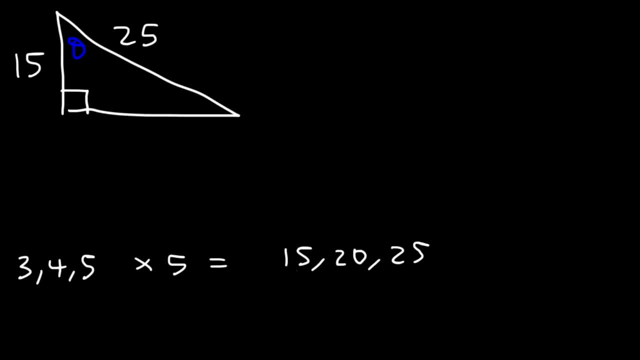 5 times 5 is 25.. So we have the 15. And we have the 25.. Therefore, the missing side must be 20.. And you can use the Pythagorean theorem to confirm this if you want to. So now let's go ahead and find the value of sine theta. 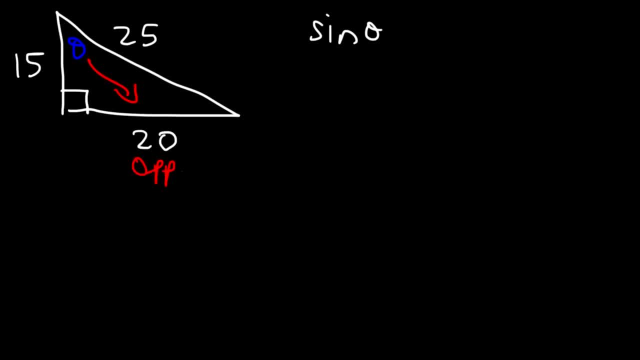 So opposite to theta is 20.. The hypotenuse is always across the box, It's the longer side. So 27 is the hypotenuse And adjacent to 15.. Right next to it is 15.. I mean adjacent to theta is 15.. 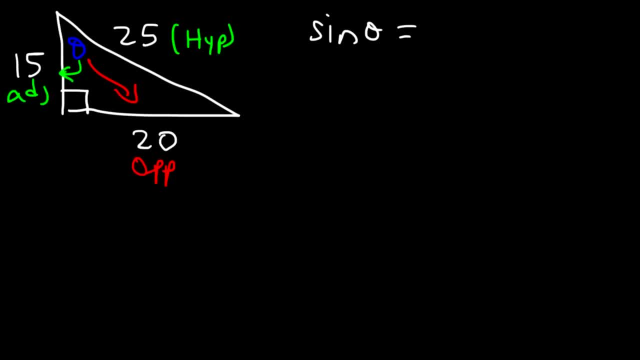 Now, sine theta, we know it's opposite, divided by hypotenuse, So it's 20 over 25.. Which reduces to 4 over 5.. If we divide both numbers by 5.. 20 divided by 5 is 4.. 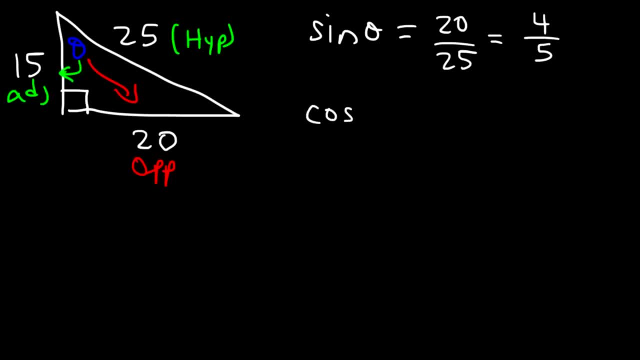 25 divided by 5 is 5.. Cosine theta is adjacent over hypotenuse. So that's 15 divided by 25.. Which reduces to 4 over 5.. Which reduces to 3 divided by 5.. Tangent theta is opposite over adjacent. 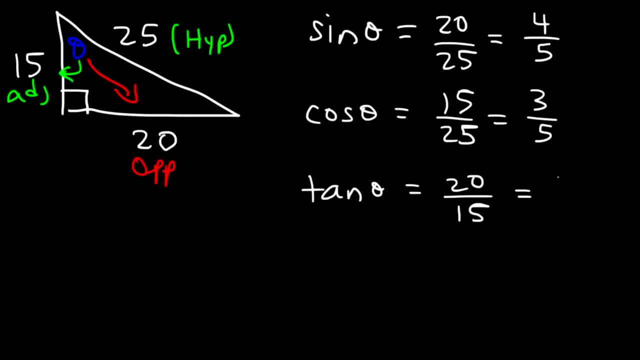 So 20 over 15.. Which becomes, If you divide by 5, that's going to be 4 over 3.. Now, cosecant is the reciprocal of sine, So it's going to be 5 over 4.. Based on this value, 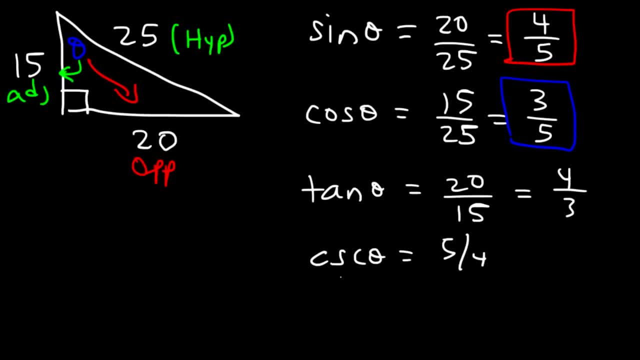 And if cosine is 3 over 5. Then secant the reciprocal of sine Has to be 5 divided by 3.. Now, if tangent is 4 over 3. Cotangent has to be 3 divided by 4.. 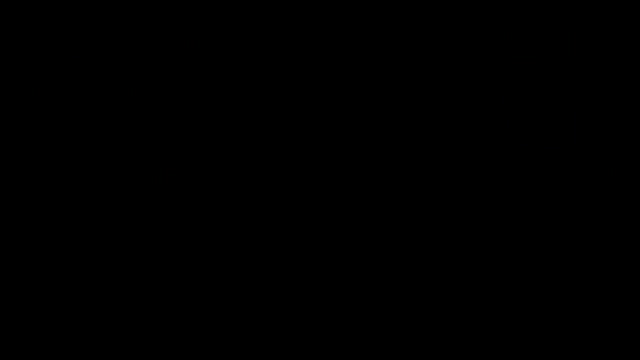 And so that's it for this problem. Consider the right triangle. In this right triangle, find the missing side, In this case, find the value of x. Let's say, the angle is 38 degrees And this side is 42.. 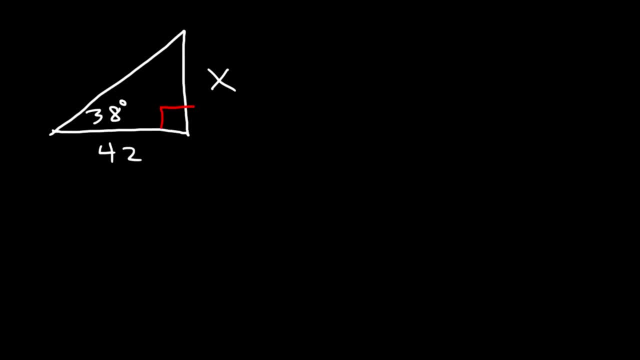 So what trig function should you use in order to find the value of x? Should we use sine cosine or tangent? Well, relative to 38, we have the opposite side, which is x, And the adjacent side, which is 42.. 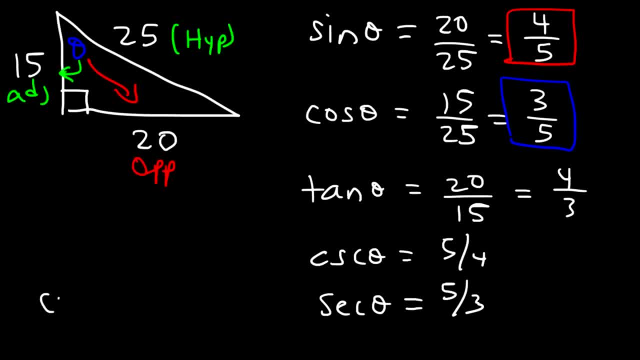 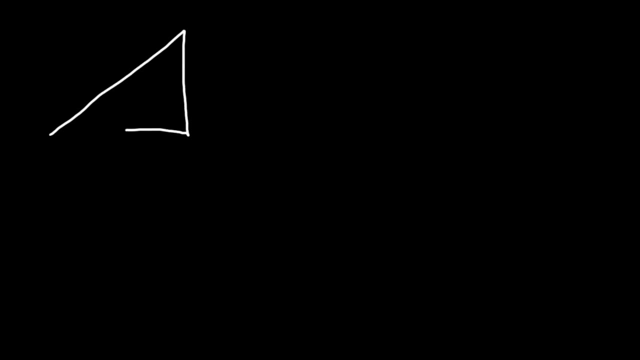 cosine has to be 5 divided by 3.. Now, if tangent is 4 over 3, cotangent has to be 3 divided by 4.. And so that's it for this problem. Consider the right triangle. In this right triangle, find the missing side. In this case, 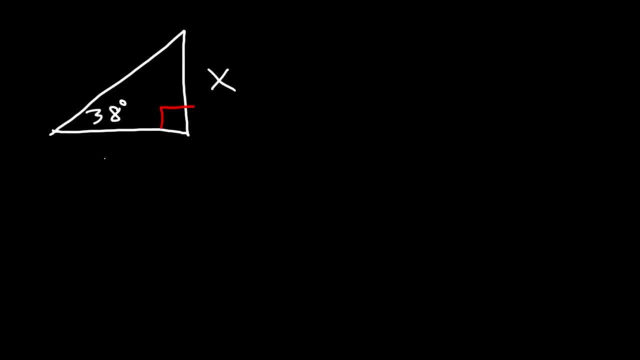 find the value of x. Let's say, the angle is 38 degrees and this side is 42. So what trig function should you use to find the missing side? Should we use sine cosine or tangent? Well, relative to 38, we have the opposite side, which is x, and the adjacent side, which. 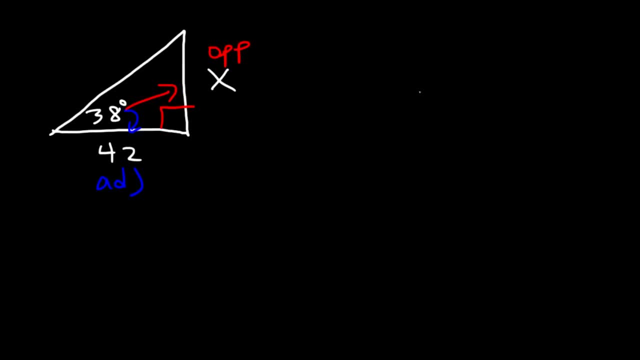 is 42. So tangent, we know it's opposite over adjacent. So therefore, tangent of the angle, 38 degrees, is equal to the opposite side, x divided by the adjacent side of 42. So in order to get x by itself, 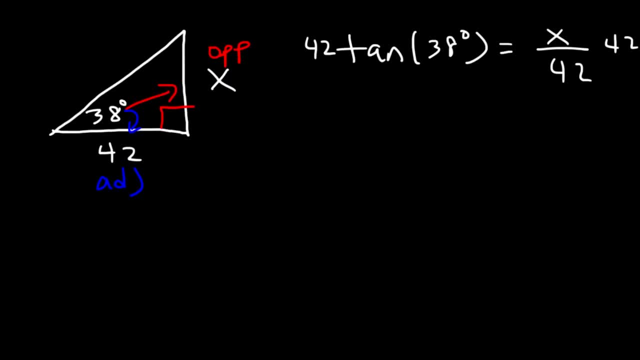 we have to multiply both sides by 42. So these will cancel. So therefore, x is equal to 42 tangent of 38. So we need to use the calculator to get this answer And make sure your calculator is in degree mode. 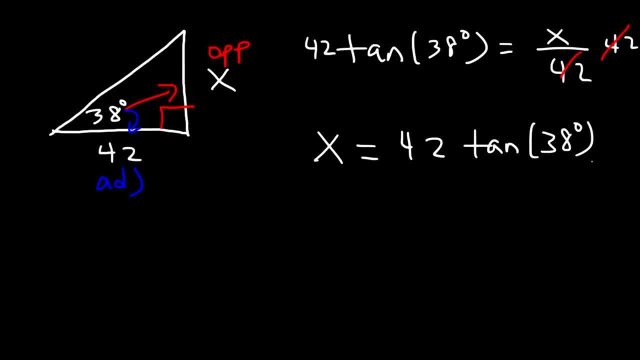 So tan 38,, which is 0.7813, and let's multiply that by 42. So this will give you an x value of 32.8.. Now let's try another example. Feel free to pause the video to work on each of these problems. by the way, 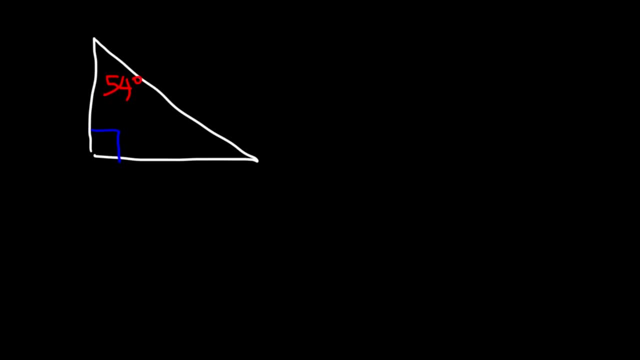 So let's say this angle is 54 degrees and we're looking for the value of x and hypotenuse is 26.. Which trig function should we use? Sine, cosine or tangent? So opposite to the right angle. we know it's the hypotenuse. 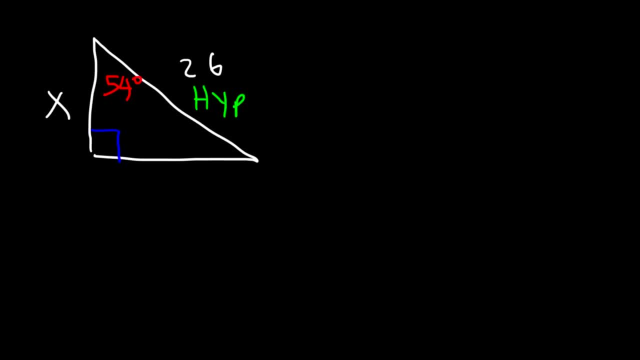 And x is on the adjacent side relative to 54. So cosine is associated with adjacent and hypotenuse. So therefore, cosine of the angle 54 is equal to the adjacent side, x divided by the hypotenuse of 26.. 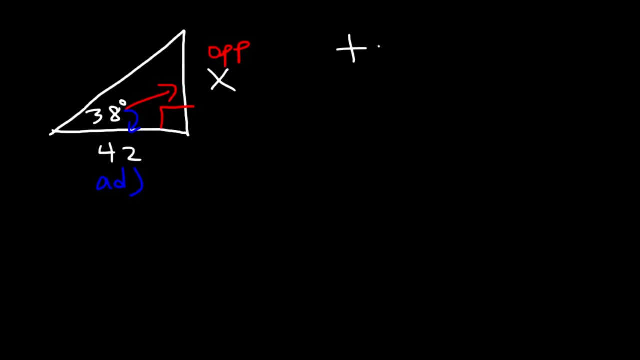 So tangent, we know it's opposite over adjacent. So therefore, tangent of the angle, 38 degrees, is equal to the opposite side: x Divided by the adjacent side. x Divided by the adjacent side, 42.. So in order to get x by itself, we need to multiply both sides by 42.. 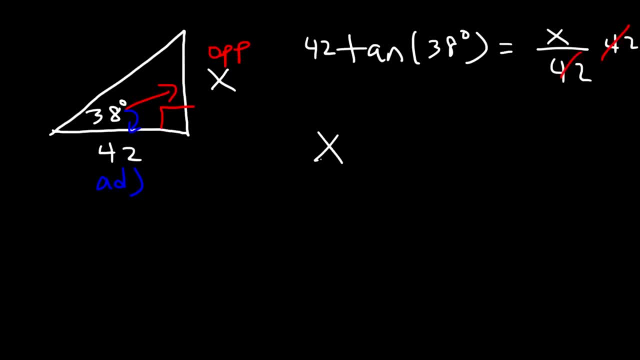 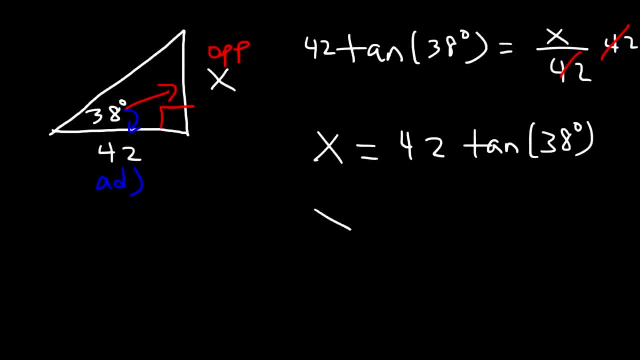 So tan 38,, which is 0.7813.. So tan 38,, which is 0.7813.. So tan 38, which is 0.7813.. And let's multiply that by 42. So this will give you an x value of 32.8.. 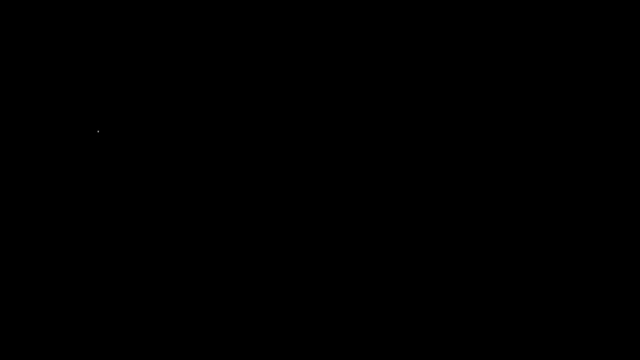 Now let's try another example. Feel free to pause the video to work on each of these problems, by the way. So let's say this angle is 54 degrees And we're looking for the value of x, And hypotenuse is 26.. 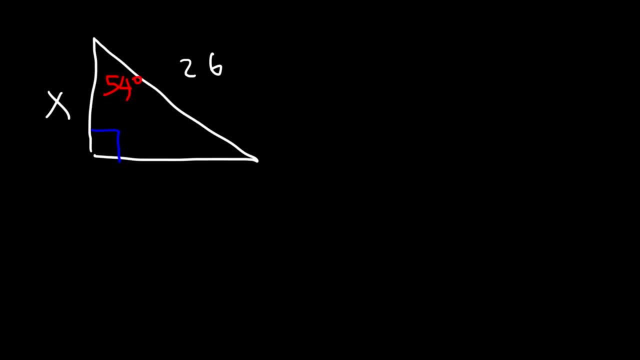 And we're looking for the value of x And we're looking for the value of x. Which trig function? should we use Sine, cosine or tangent? So opposite to the right angle. we know it's the hypotenuse. 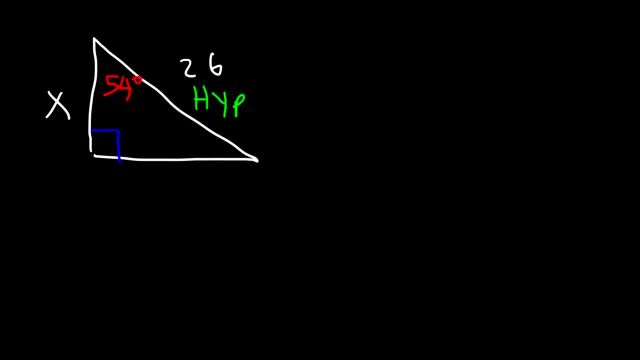 And x is on the adjacent side relative to 54. So cosine is associated with adjacent and hypotenuse. So therefore cosine of the angle 54 is equal to the adjacent side x divided by the hypotenuse of 26.. So to get x by itself we've got to multiply. 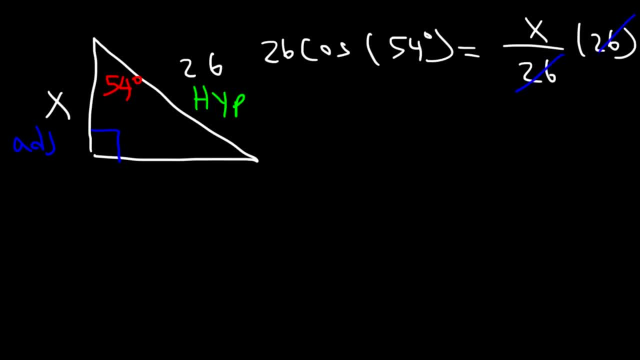 We've got to multiply both sides by 26.. So therefore, x is equal to 26. cosine of 54 degrees, Cosine 54 is 0.587785.. If we multiply that by 26,, this will give us the value of x, which is 15.28.. 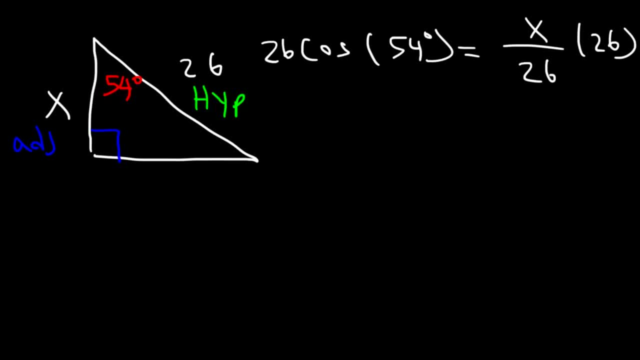 So to get x by itself we've got to multiply both sides by 26.. So therefore x is equal to 26, cosine of 54 degrees. Cosine 54 is .587785.. If we multiply that by 26,, this will give us the value of x, which is 15.28.. 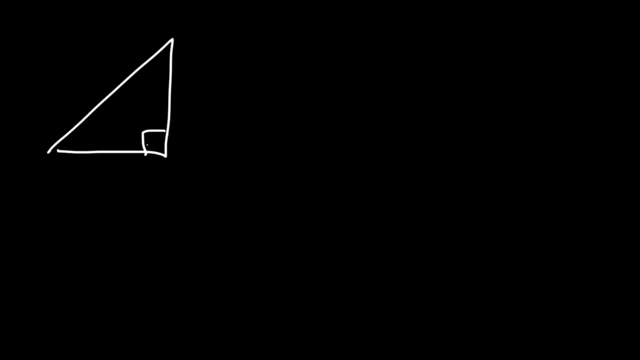 Here's another one that we could try. Let's say the angle is 32 degrees and the hypotenuse is x, and this is 12.. So notice that 12 is opposite to 32, and we have the hypotenuse. 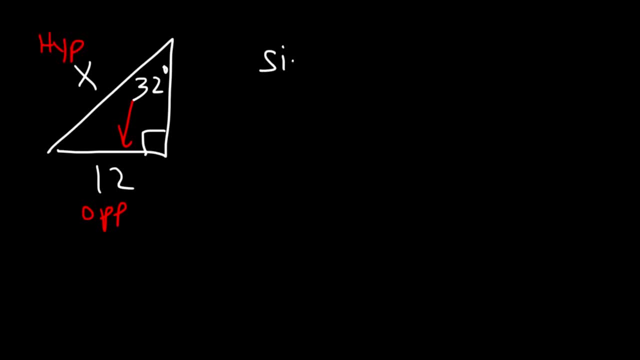 So this time we need to use the sine function. Sine of the angle 32 is equal to the opposite side, 12, divided by x. So in this case, what can we do? So in this case, what can we do? 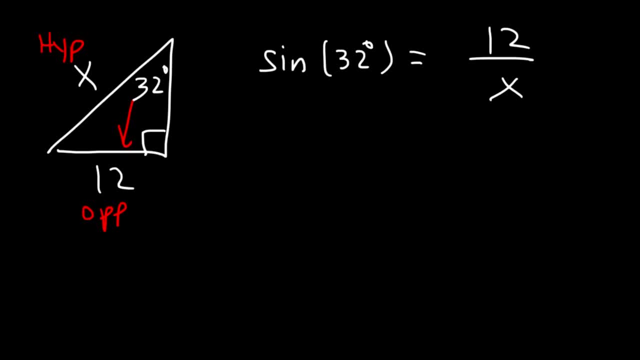 So, in this case, what can we do? What can we do to find the value of x? What would you do? What I would do is cross multiply. So 1 times 12 is 12, and this is going to equal x times sine 32.. 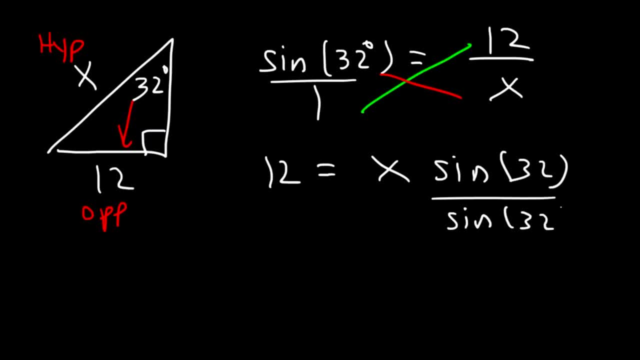 Next, I recommend dividing both sides by sine 32.. Sine 32 divided by itself is 1.. So therefore x is equal to 12 over sine 32.. 12 divided by sine 32 is 22.64.. 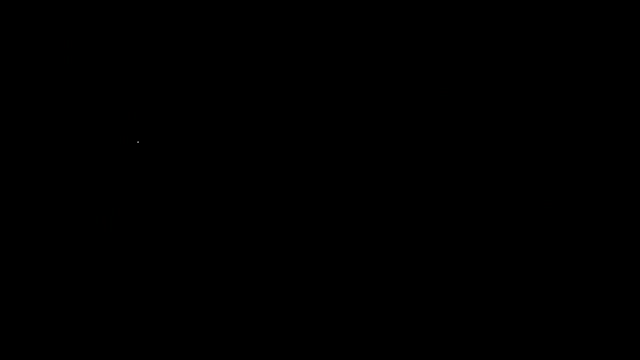 So that's the value of x in this particular problem. Now let's work on another problem. So this time we need to find the angle theta, And we're given these two sides. So 5 is opposite to the angle and 4 is adjacent to it. 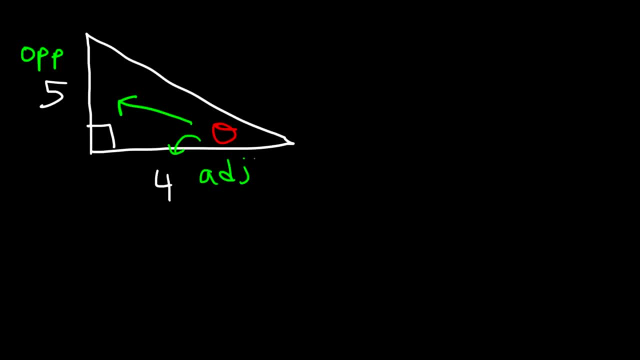 So what trig function can relate theta 4, and 5?? We know tangent is opposite over adjacent. So tangent of the angle theta is equal to the opposite side, which is 5, divided by the adjacent side, 4.. 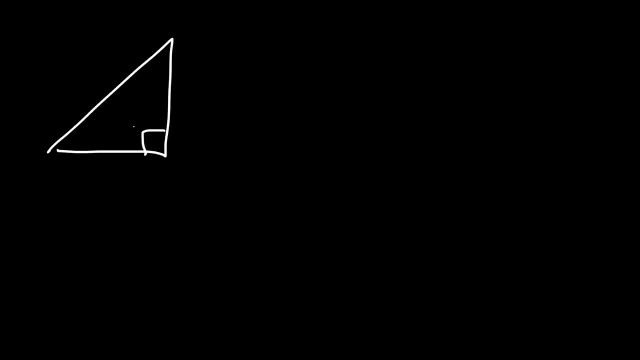 Here's another one that we could try. Let's say the angle is 32 degrees And the hypotenuse is x, And this is 12.. So notice that 12 is opposite to 32.. And we have the hypotenuse. 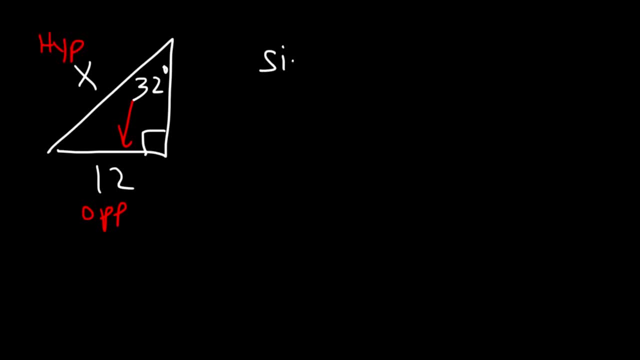 So this time we need to use the sine function. Sine of the angle 32 is equal to the opposite side, 12 divided by x. So in this case, what can we do to find the value of x? What would you do? 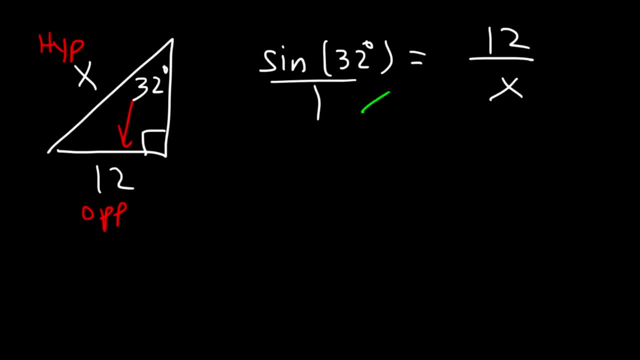 What I would do is cross multiply. So 1 times 12 is 12.. And this is going to equal x times sine 32.. Next, I recommend dividing both sides by sine 32.. Sine 32 divided by itself is 1.. 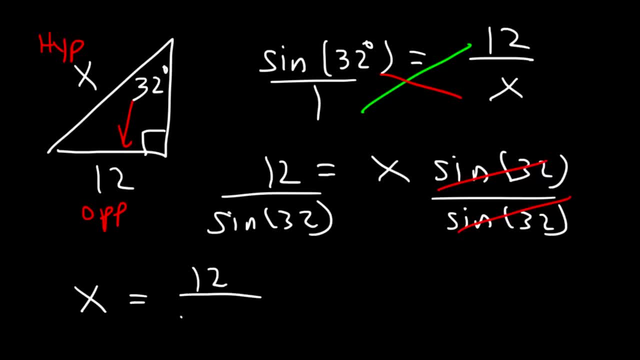 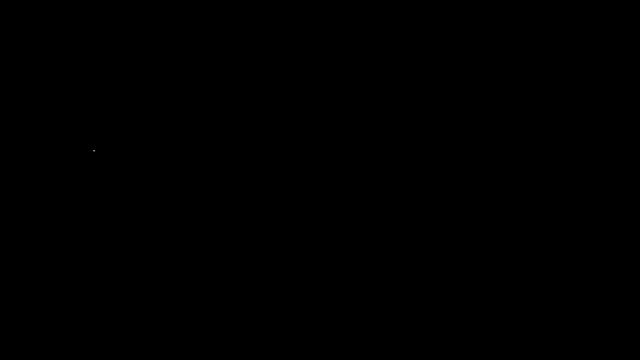 So therefore x is equal to 12 over sine 32.. 12 divided by sine 32 is 22.64.. So that's the value of x in this particular problem. Now let's work on another problem. So this time we need to find the angle. 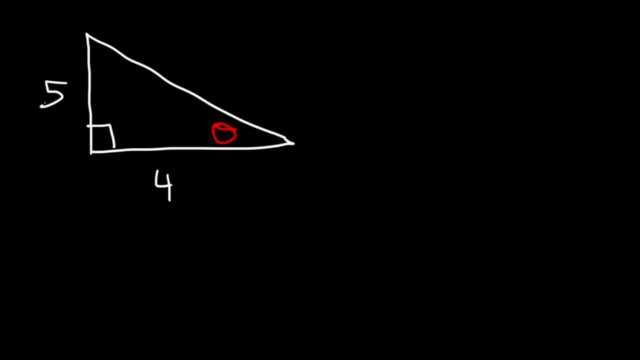 theta and we're given these two sides. So 5 is opposite to the angle and 4 is adjacent to it. So what trig function can relate theta 4 and 5?? We know tangent is opposite over adjacent. so tangent of the angle theta is equal to the opposite. 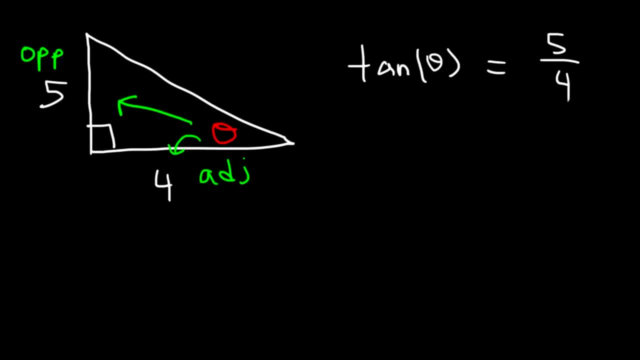 side, which is 5 divided by the adjacent side, 4.. So how can we find the value of the angle theta? If tangent theta is 5 over 4, then theta is going to be the inverse tangent or arctangent of 5 over 4, and you simply have to type this in. 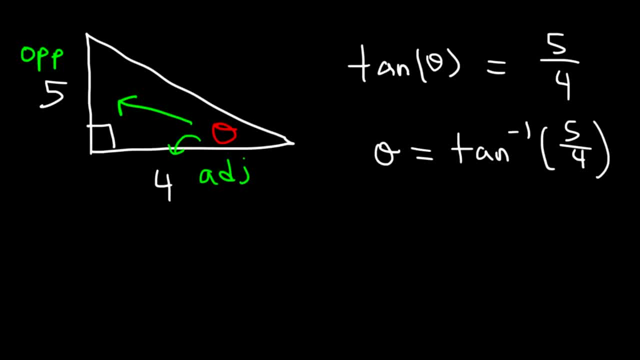 your calculator. So type in arctan 5 over 4 and you should get an angle of 51.34 degrees. So that's how you could find the missing angle. Let's try another example. Feel free to pause the video and find the missing angle. So in this case we have the. 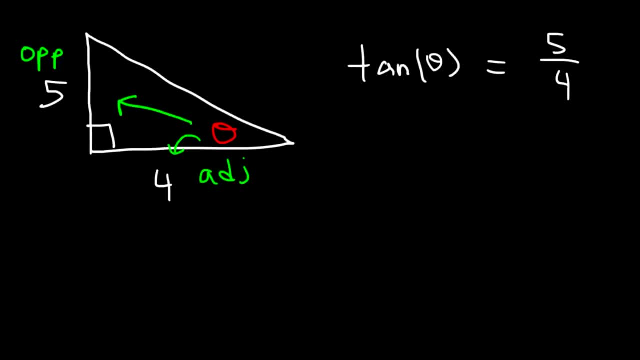 So how can we find the value of theta? If tangent theta is 5 over 4, then theta is going to be the inverse tangent or arctangent of 5 over 4.. And you simply have to type this in your calculator. 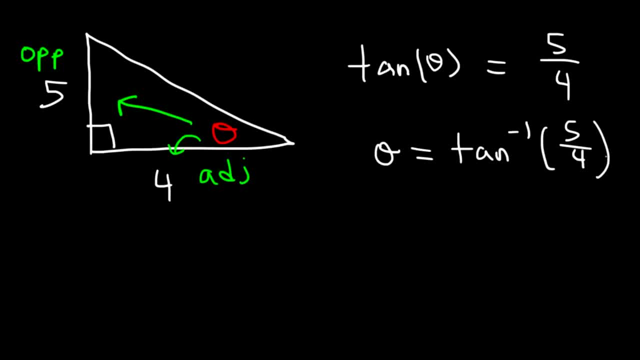 So type in arctan 5 over 4. And you should get an angle of 51.34 degrees. So that's how you can find the missing angle. Let's try another example. Feel free to pause the video and find the missing angle. 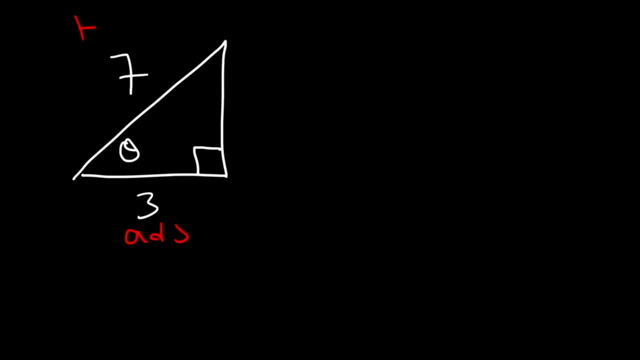 So in this case we have the adjacent side and we have the hypotenuse. So therefore this is associated with cosine. Cosine theta is equal to the adjacent side divided by the hypotenuse. So if cosine theta is equal to 3 divided by 7, theta is going to be arctosine 3 over 7.. 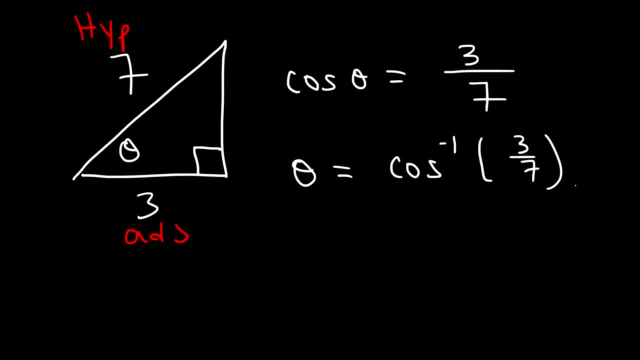 And once again you have to find the missing angle. So you have to use a calculator to figure this out, Because without a calculator, how do we know what this answer is? And this is going to be 64.62 degrees. 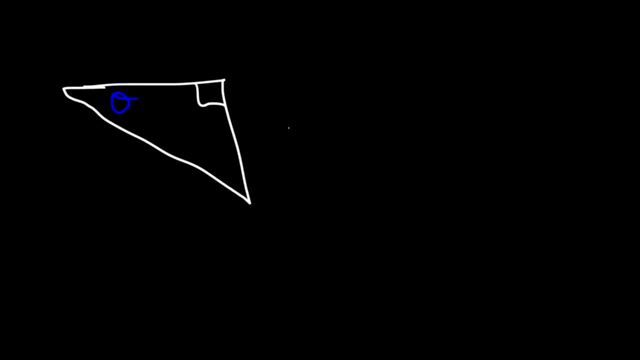 So here's another one for you. Let's say this is 5 and this is 6. Go ahead and find the value of theta. So the hypotenuse is 6.. Opposite to theta is 5.. So we know sine is associated with opposite and hypotenuse. 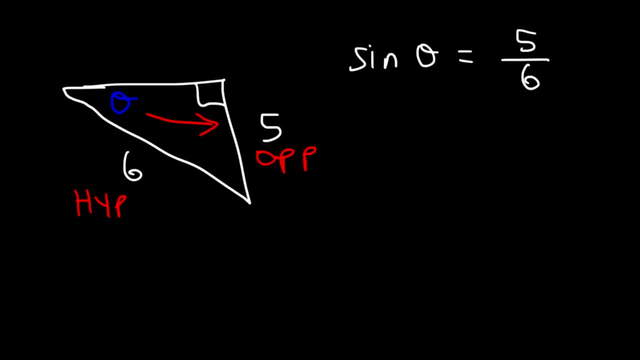 Sine, theta is equal to the opposite side, which is 5, divided by the hypotenuse, which is 6.. Therefore, theta is the arcsine, or inverse sine of 5 over 6.. And so the angle is going to be 56.44 degrees. 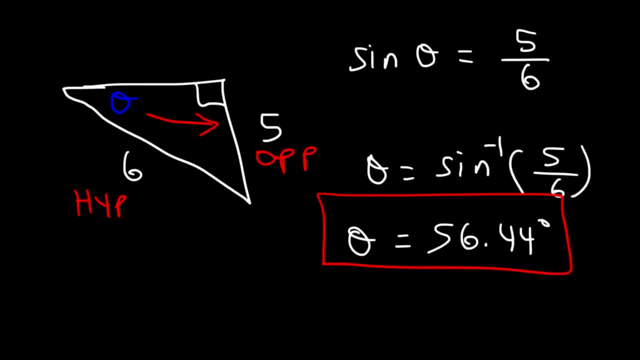 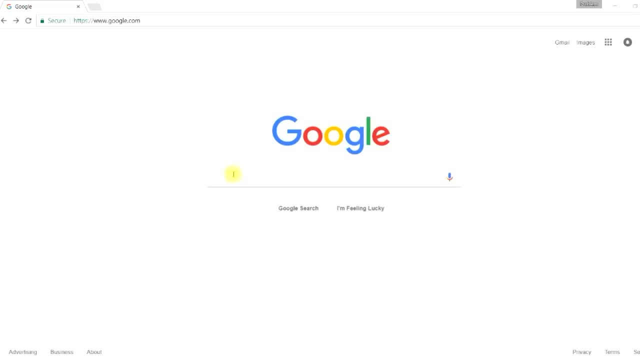 And that's it. That's all you've got to do to find the missing angle of a right triangle. So that's it. For those of you who might be interested in my trigonometry course, here's how you can access it. 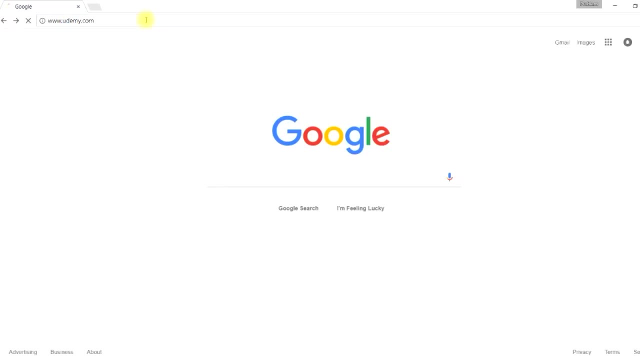 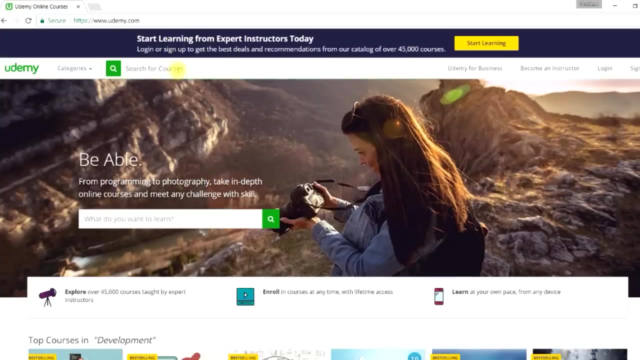 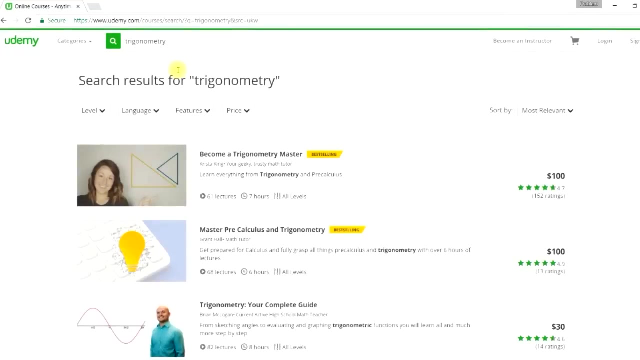 So go to udemycom And, once you're there, enter into the search box trigonometry. Now, this is a course I've recently created, so I haven't finished adding all the sections that I want to add, So in time I'm going to do that. 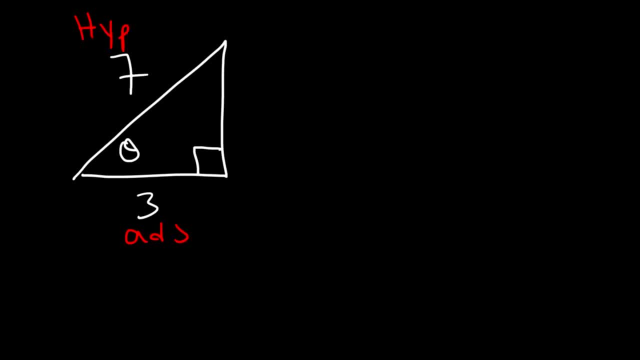 adjacent side and we have the hypotenuse. So therefore this is associated with cosine. Cosine theta is equal to the adjacent side divided by the hypotenuse. So if cosine theta is equal to 3 divided by 7, theta is going to be arc cosine 3 over 7.. Once again you have to use a calculator to 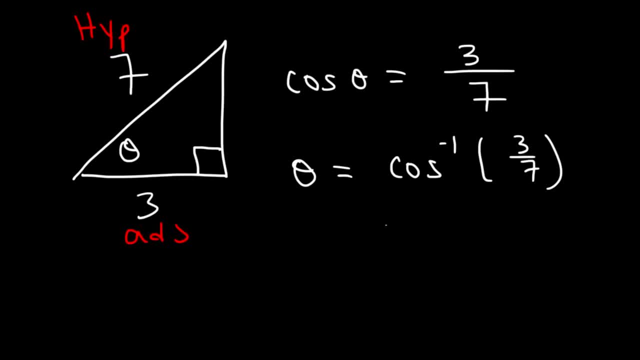 figure this out, because without a calculator, how do we know what this answer is? And this is going to be 64.62 degrees. So here's another one for you. Let's say this is 5 and this is 6.. Go ahead and find. 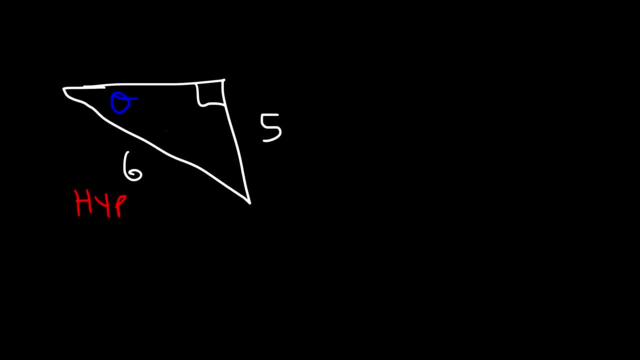 the value of theta, So the hypotenuse is 6.. Opposite to theta is 5.. So we know sine is associated with opposite and hypotenuse Sine. theta is equal to the opposite side, which is 5 divided by the hypotenuse, which is 6.. Therefore, theta is the arc, sine or inverse. 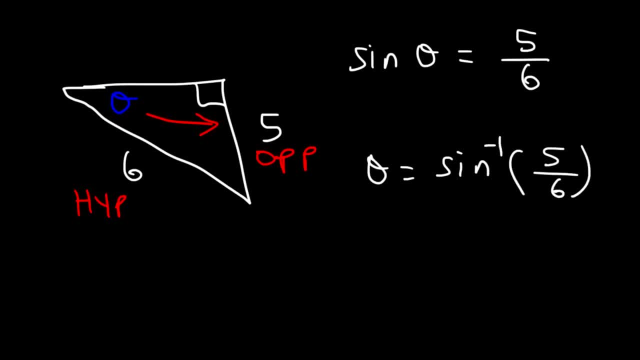 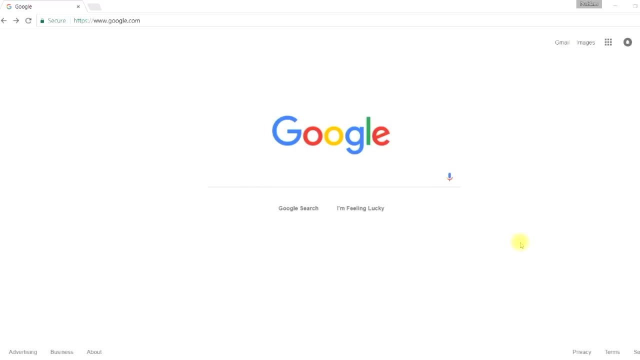 sine of 5 over 6.. And so the angle is going to be 56.44 degrees, And that's it. That's all you got to do to find the missing angle of a right triangle. For those of you who might be interested in my trigonometry course, here's how you can. 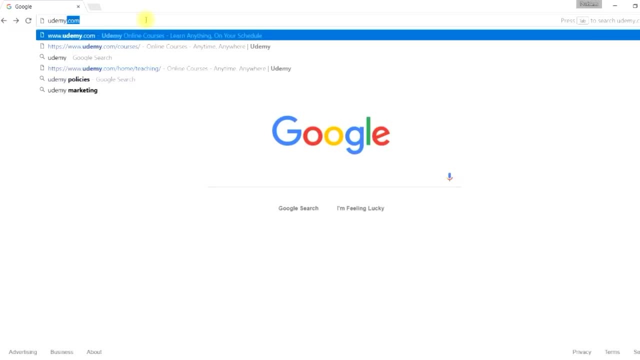 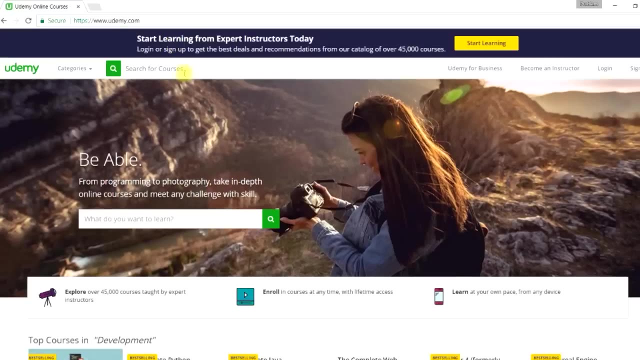 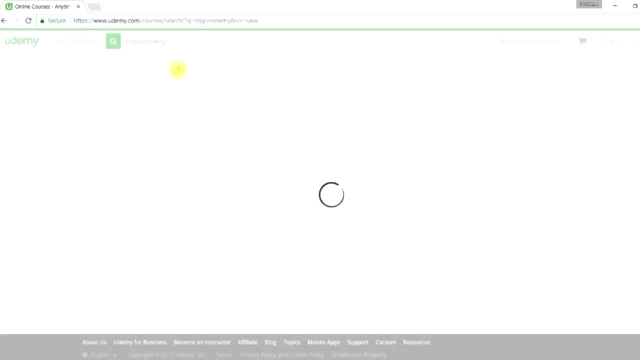 access it. So go to udemycom and once you're there, enter into the search box: trigonometry. Now, this is a course I've recently created, So I haven't finished adding all the sections that I want to add. So in time I'm going to 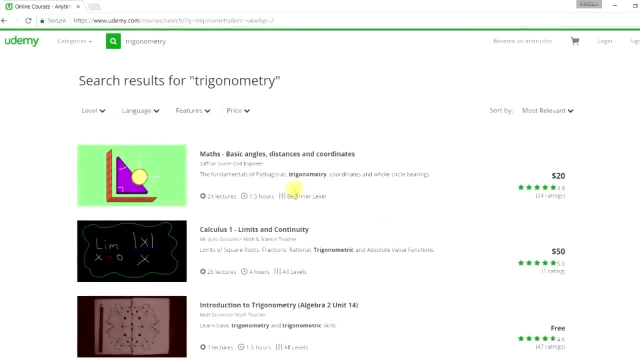 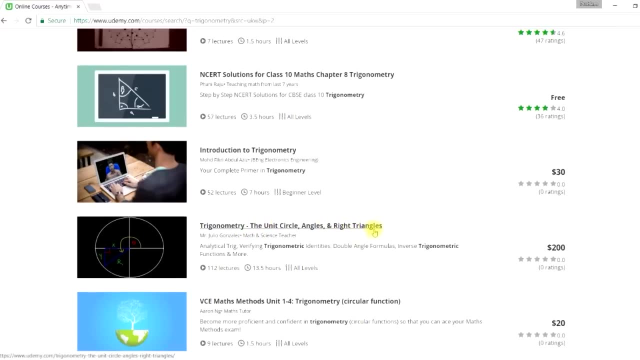 do that Right now. the page is accessible on the. you can find the course on the second page, And here it is: Trigonometry, the unit, circle, angles and right triangles. It's basically the one with the dark background and a circle with a triangle inside the circle. 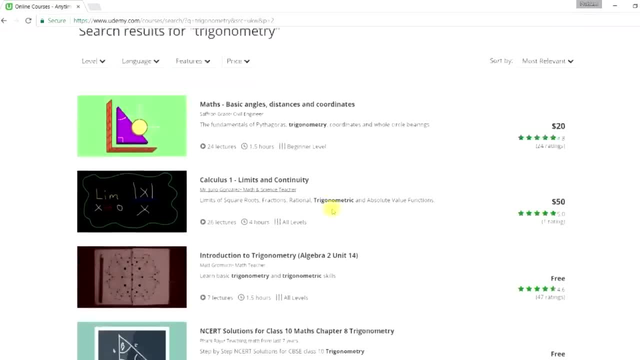 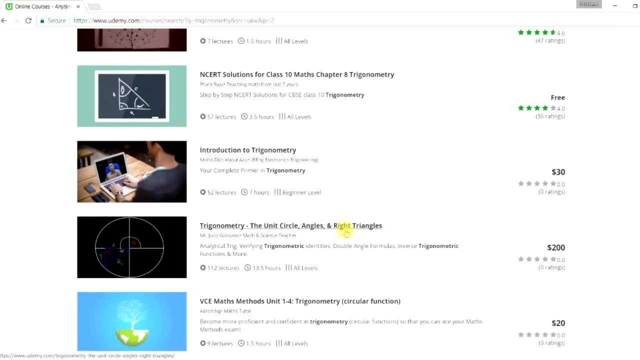 So right now the page is accessible on the uh. you can find the course on the second page, And here it is: Trigonometry, the unit circle, angles and right triangles. It's basically the one with the dark background and the circle with the triangle inside the circle. 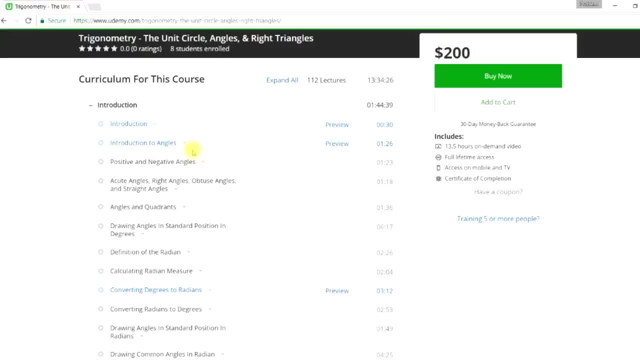 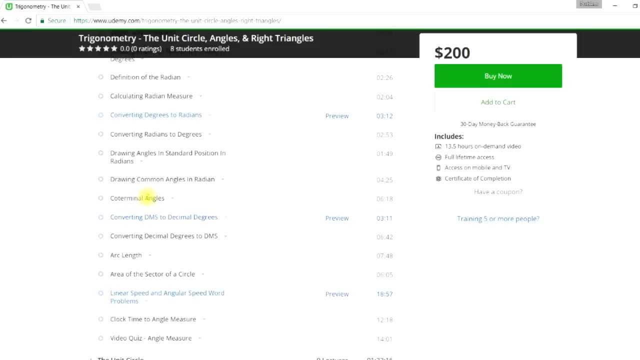 So let's look at the curriculum. In the first section I'm going to go over angles: radians- How to convert degrees to radians. Cold terminal angles. How to convert DMS to decimal degrees. Arc length- Area of the sector of a circle. 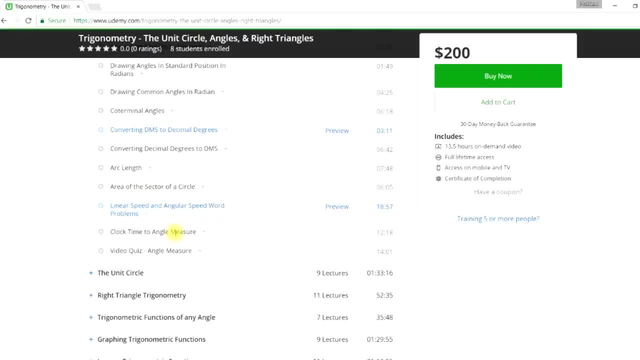 Linear speed and angular speed, word problems And also if you need to take the time that's shown on the clock and if you need to convert it to an angle measure. I cover that in this section as well, And then at the end of each section is a video quiz. 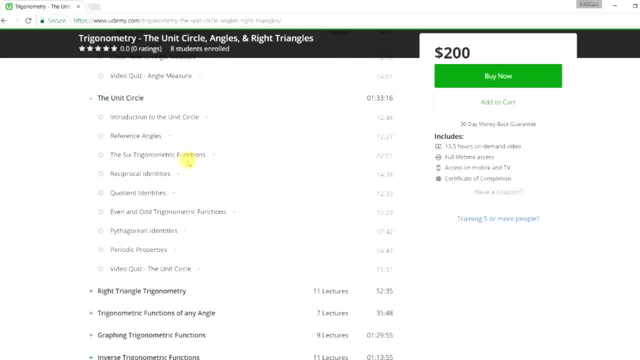 The next section is about the unit circle, The six trig functions, Sine, Cosine, Tangent, Secant, Cosecant, Cotan And also reference angles as well. After that you have right triangle trigonometry. 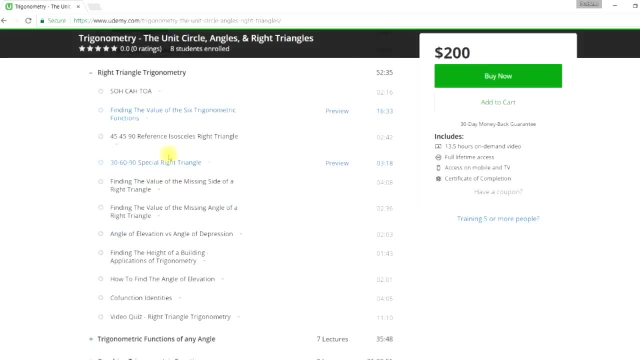 Things like SOHCAHTOA, The special right triangles like the 30,, 60, 90 triangle. You need to know that so you can evaluate sine and cosine functions without using the unit circle. Next, I'm going to talk about how to solve angle of elevation and depression problems. 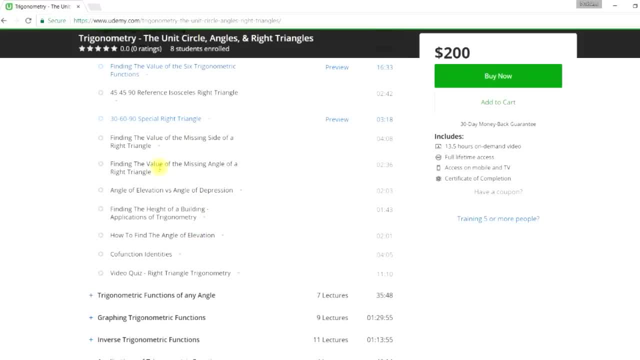 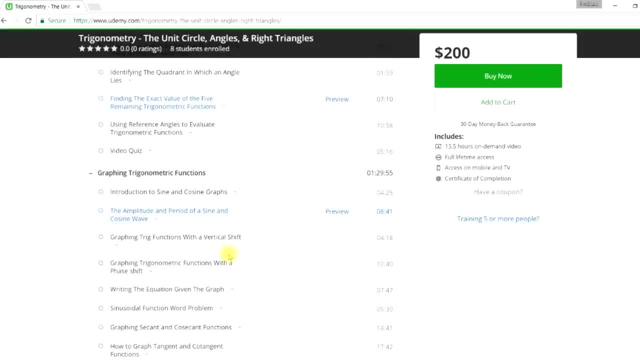 And just solving the missing sides of right triangles, After that trigonometric functions of any angle And then graphing trig functions. You need to know how to graph the sine and cosine functions, Secant, cosecant and tangent as well. 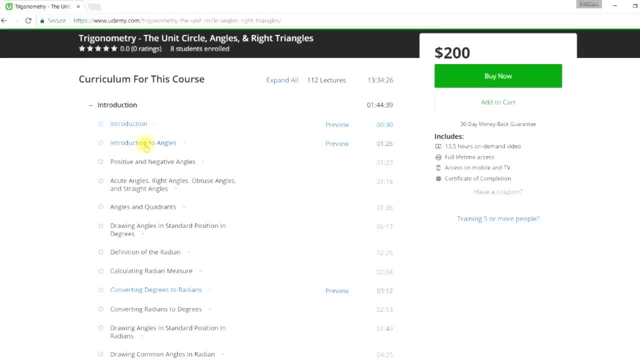 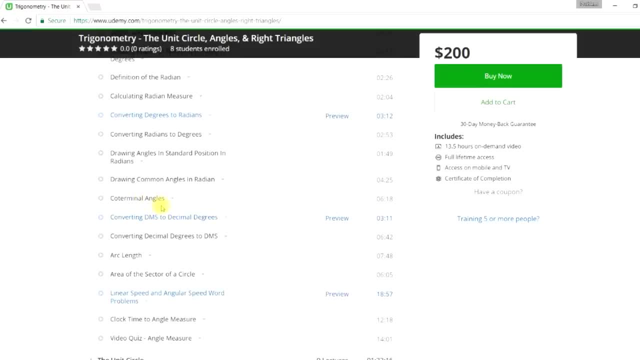 So let's look at the curriculum. In the first section I'm going to go over angles, radians, how to convert degrees to radians, coterminal angles, how to convert DMS to decimal degrees, arc length, area of the sector of a circle, linear speed and angular speed. word problems and also, if you need, 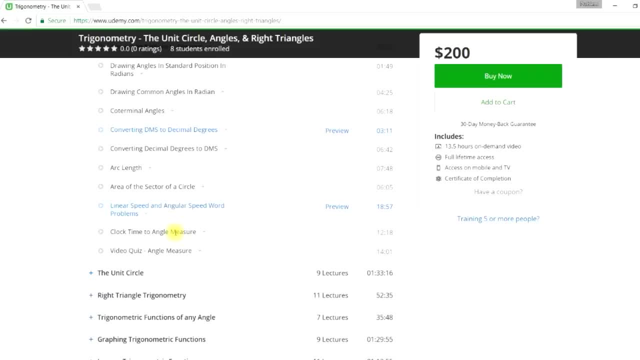 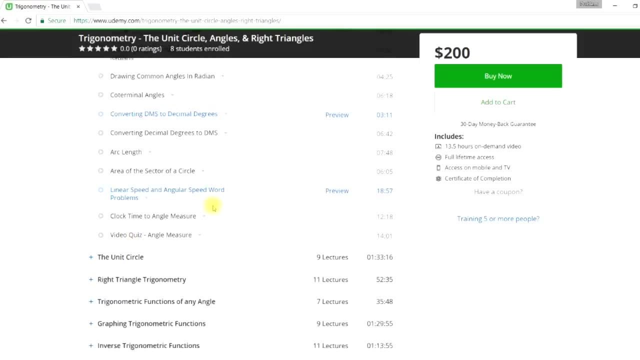 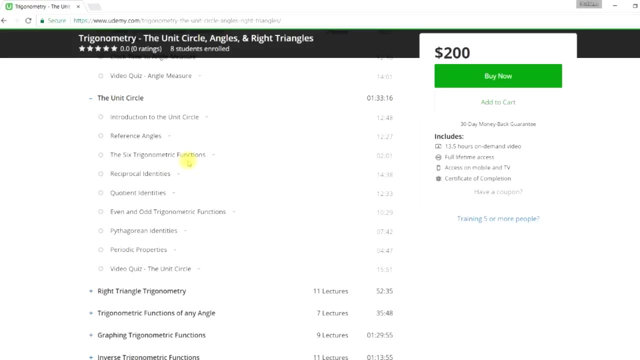 to take the time that's shown on the clock and if you need to convert it to an angle measure. I cover that in this section as well, And then at the end of each section is a video quiz. The next section is about the unit circle, The six trig functions sine cosine tangent. 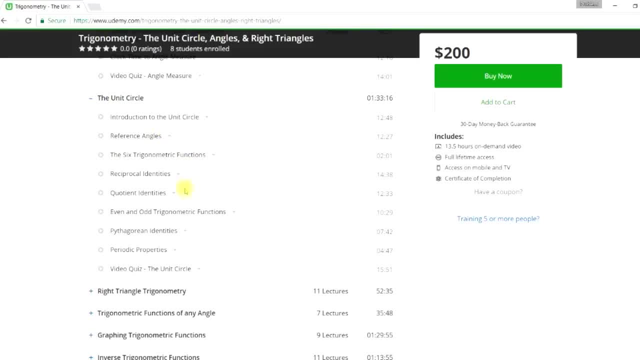 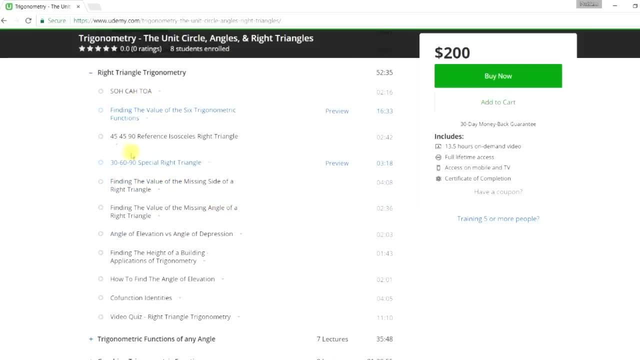 secant, cosecant, cotan, and also reference angles as well. After that you have right triangle trigonometry, things like SOHCAHTOA, the special right triangles like the 30,, 60, 90 triangle. You need to know that so you can evaluate sine and cosine functions without 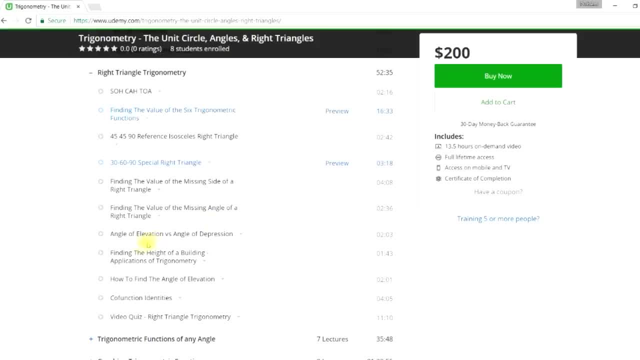 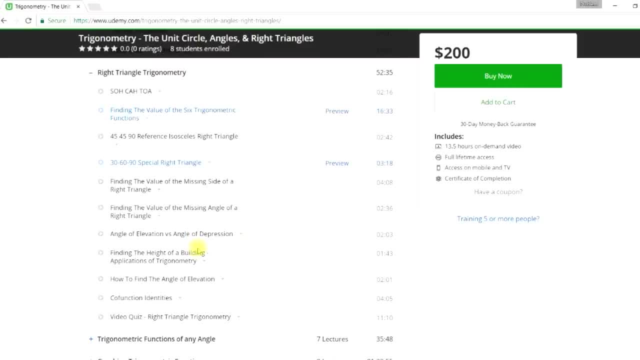 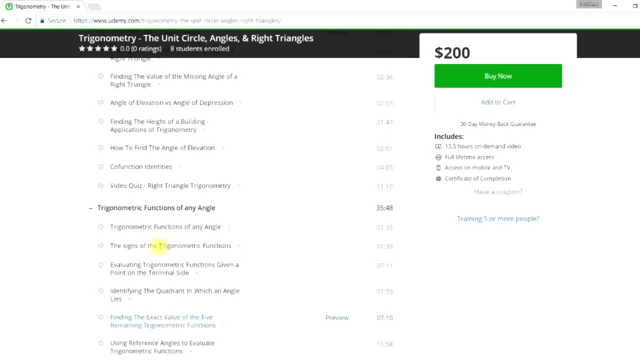 On the right we are going to talk about how to solve angle of elevation and depression problems and just solving the missing sides of right triangles. After that trigonometric functions of any angle and then you graph and trig functions. You need to know how to. 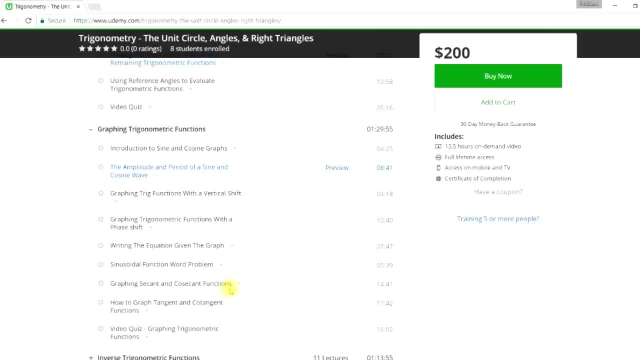 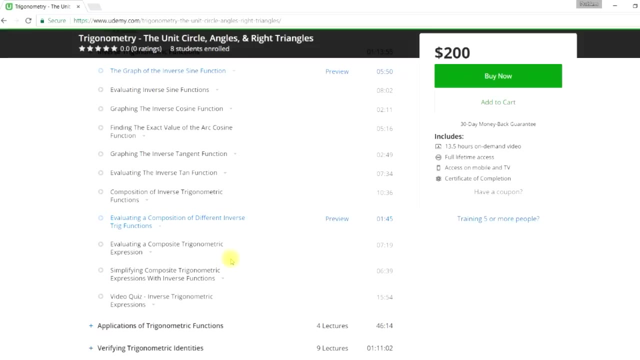 graph the sine and cosine functions, secant, cosecant and tangent as well, After that inverse trig functions. You need to know how to evaluate it, and then you have it, and also how to graph it too. In addition, you need to know how to graph or evaluate. 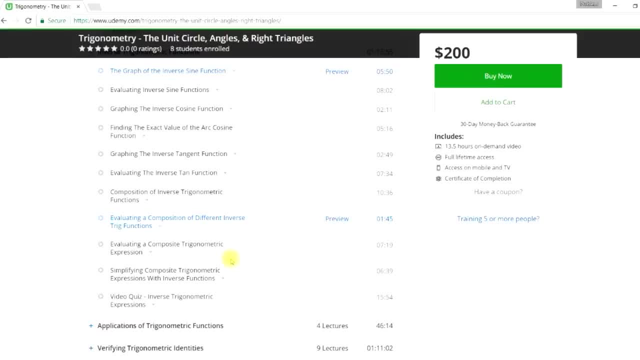 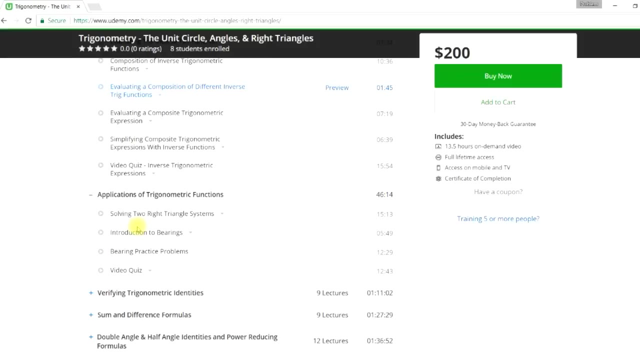 composition of trig functions. For example, you might have sine of inverse, cosine of 3 over 4, something like that, And you can use the right triangle to solve those types of problems. You'll see it when you access that section After that. applications of trig functions: solving problems. 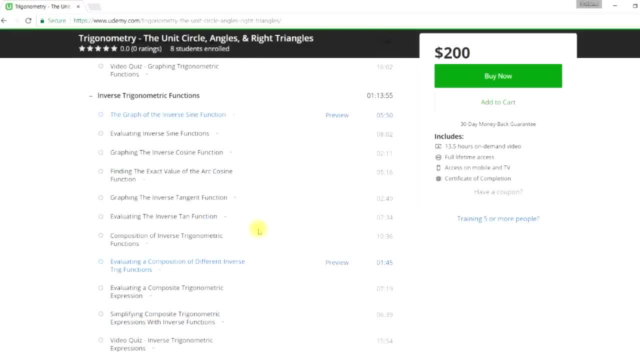 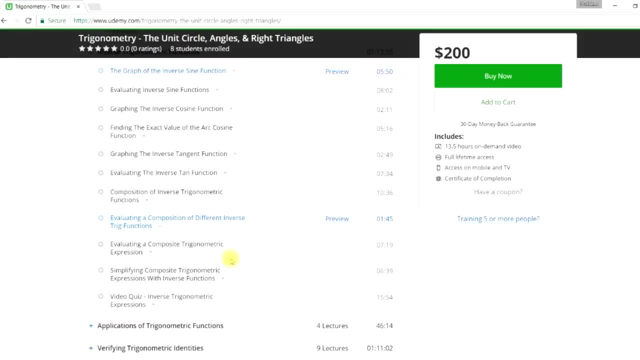 After that, inverse trig functions. You need to know how to evaluate it And also how to graph it too. In addition, you need to know how to graph. You need to know how to graph or evaluate composition of trig functions. For example, you might have sine of inverse cosine of 3 over 4 or something like that. 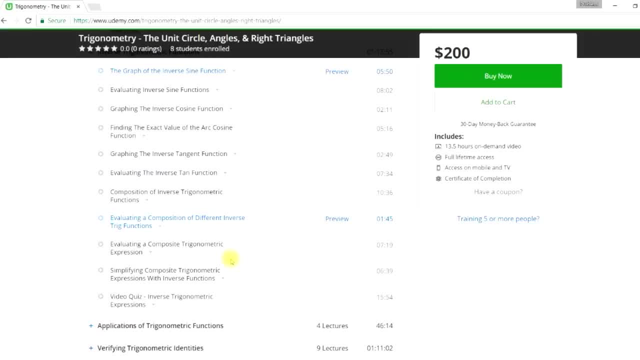 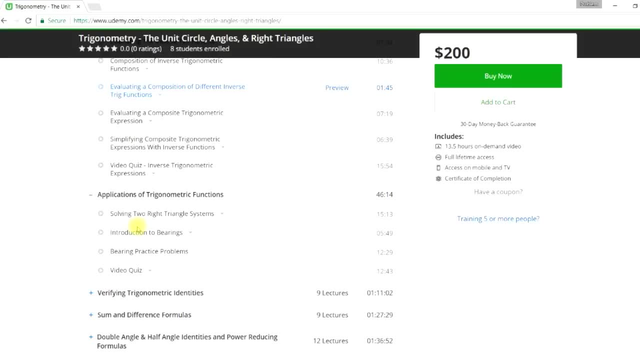 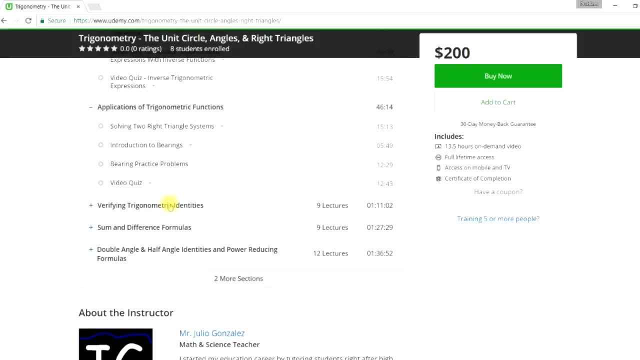 And you can use the right triangle to solve those types of problems. You'll see it when you access that section. After that, applications of trig functions Solving problems that have two right triangles in it, And barons as well. One of the hardest sections in trig is this section. 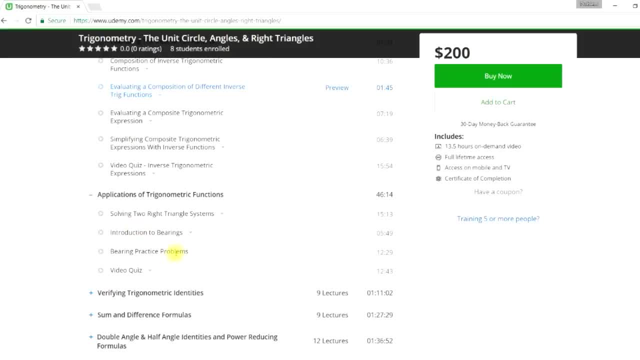 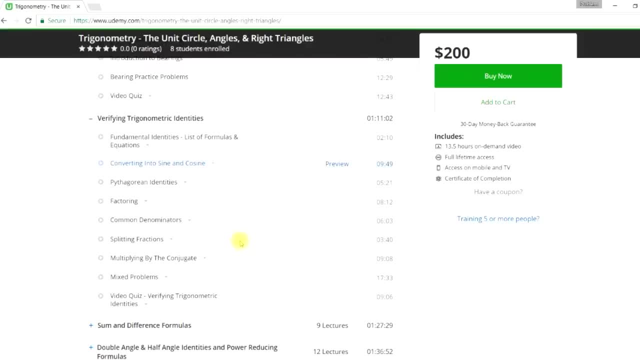 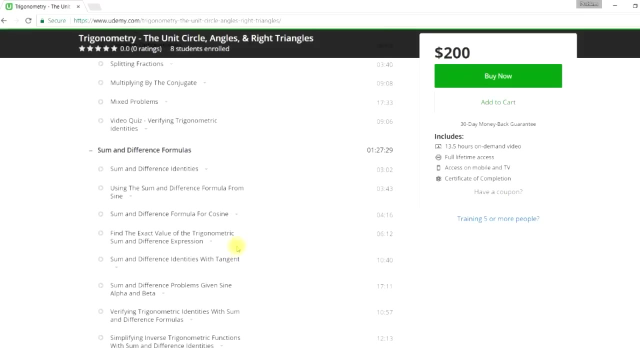 that have two right triangles in it, and Barron's as well. One of the hardest sections in trig is this section, verifying trig identities. So that's a hard one, so make sure you spend some time learning that section. After that, sum and difference formulas: double angle, half angle. 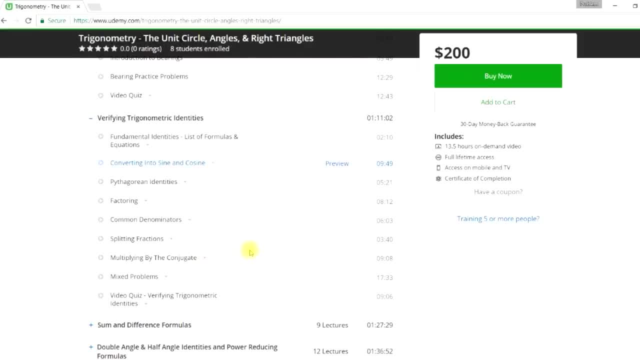 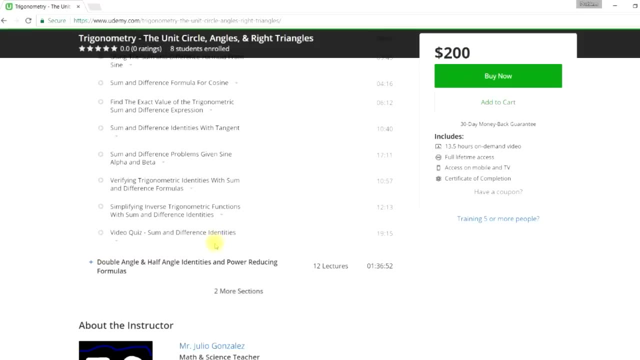 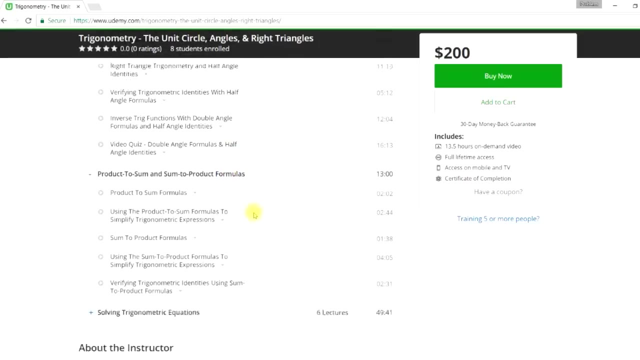 Verifying trig identities. So that's a hard one, So make sure you spend some time learning that section After that. sum and difference formulas: Double angle, half angle, power, reducing formulas: Product to sum, sum to product. 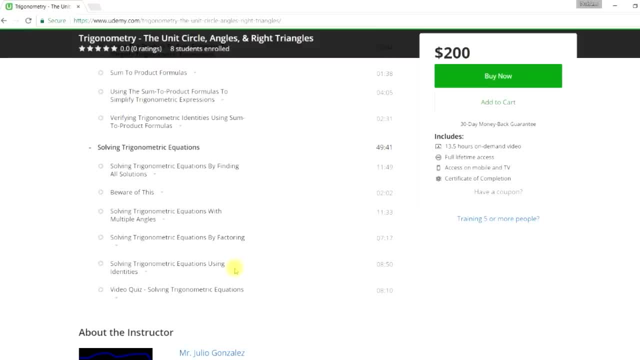 And also solving trig equations. But there are still some sections I'm going to add to this course, Like, for example, law of sines, law of cosines, polar coordinates and some other topics as well. So about two-thirds of the course is finished so far. 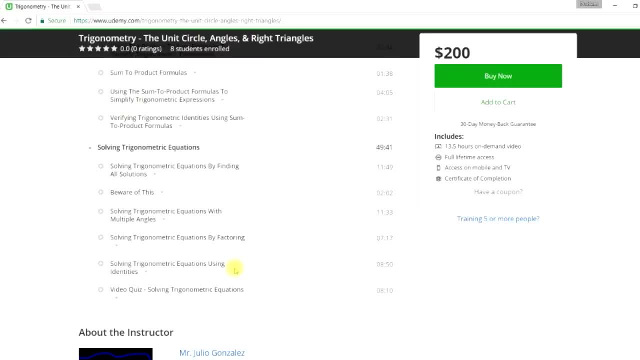 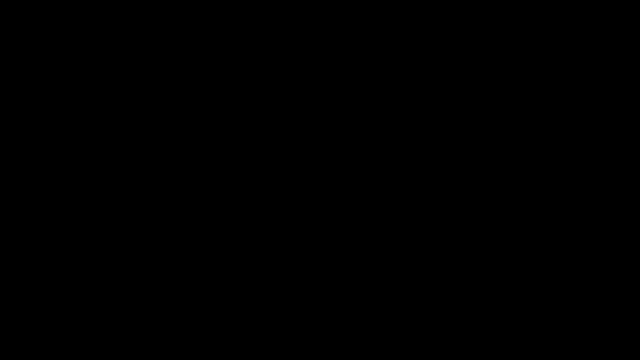 And for most students this is just what they need in trig, But in time you'll see more. So now you know how to access the course And if you have any questions, let me know. So thanks for watching. 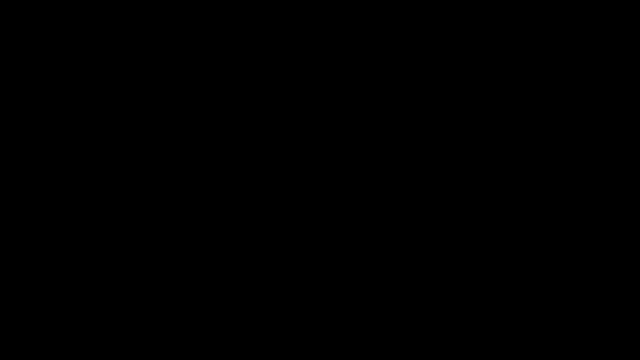 Subtitles by the Amaraorg community.